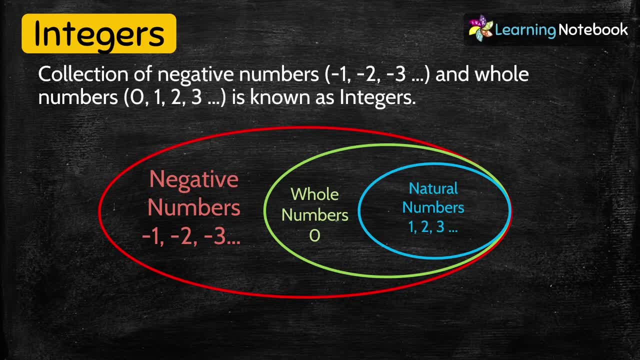 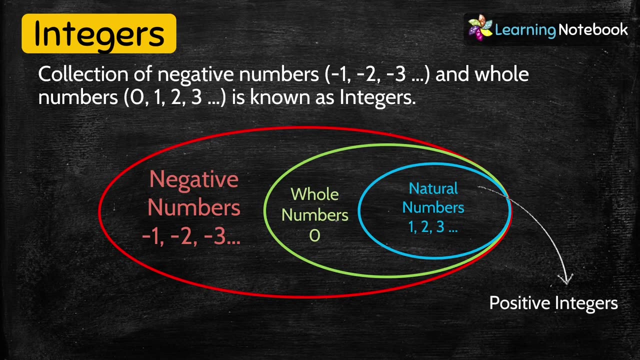 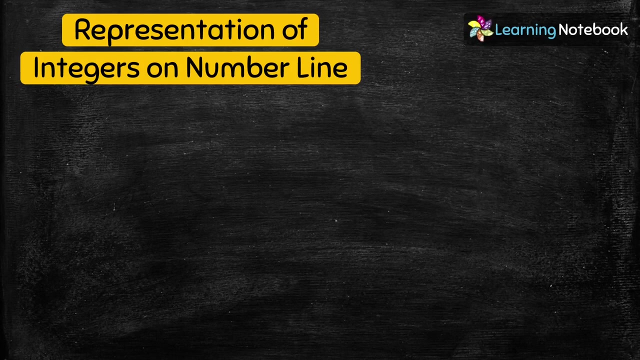 So, students, collection of negative numbers And whole numbers is known as integers. Natural numbers are called as positive integers And negative numbers are called as negative integers. Let's move to next topic: Representation of integers on number lines. Students, let's look at this number line. This number line is divided into two parts. 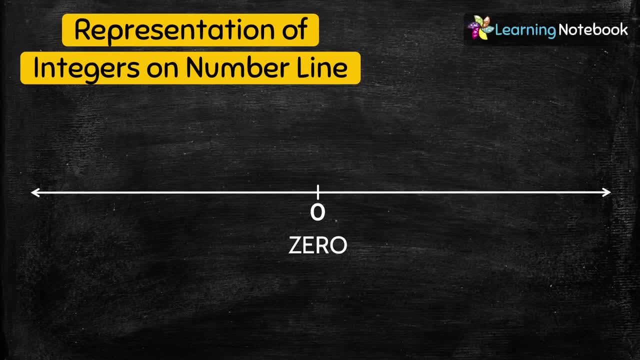 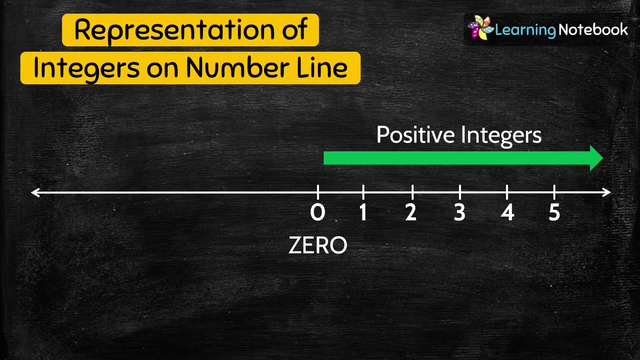 Left part and right part by the number 0. 0 is the integer which is neither negative nor positive. The numbers on the right side of the 0 are the positive integers. These positive integers can be written with or without positive sign, While the numbers on the left side of the 0 are the negative integers. 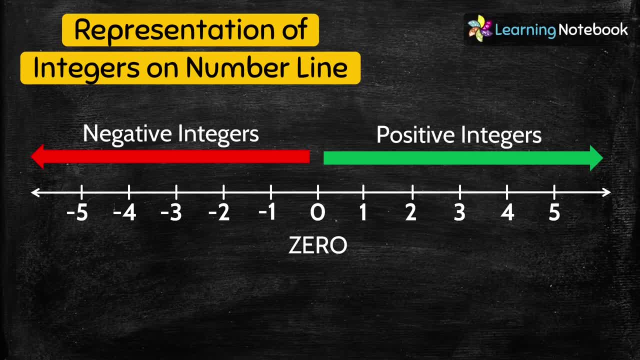 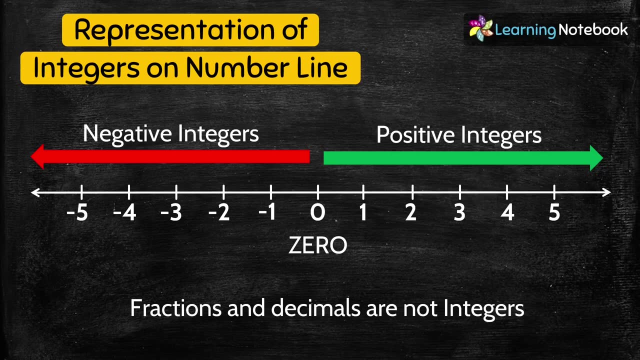 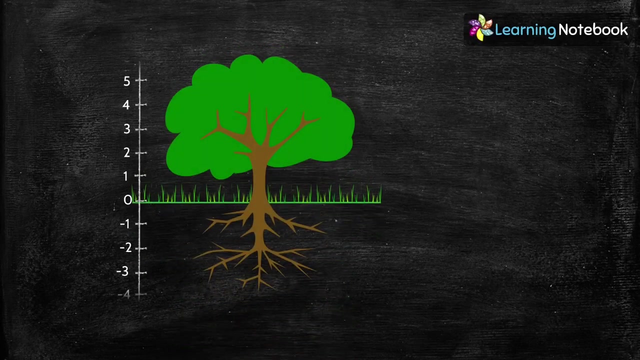 These negative integers must be written with negative sign. Students do remember that fractions and decimals are not integers. Now let's see some real world situations which can be described by integers. Take a look at this tree. The ground level represents 0.. Below the ground level represents: 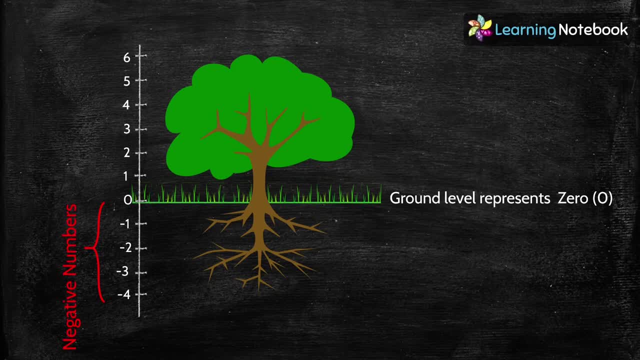 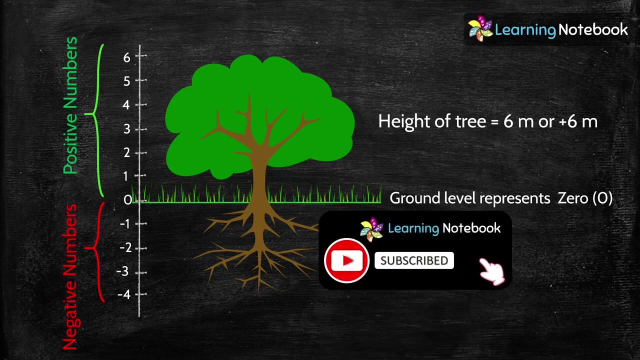 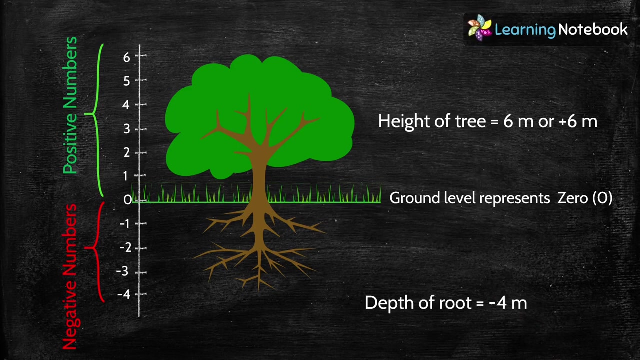 negative numbers and above the ground level represents positive numbers. So if we say the height of the tree is 0, then the value of the tree must be zero. middle of the tree is 6 meters, it is equivalent to positive 6.. And if we say depth of the root is 4 meters, 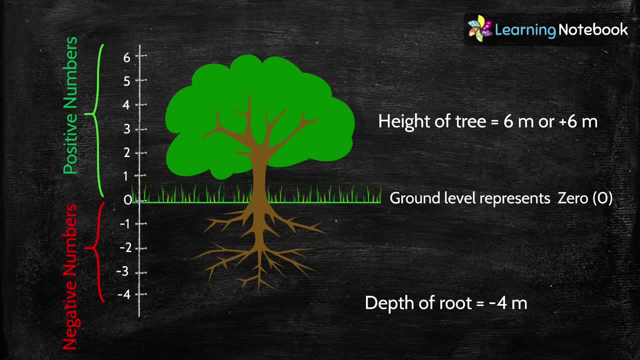 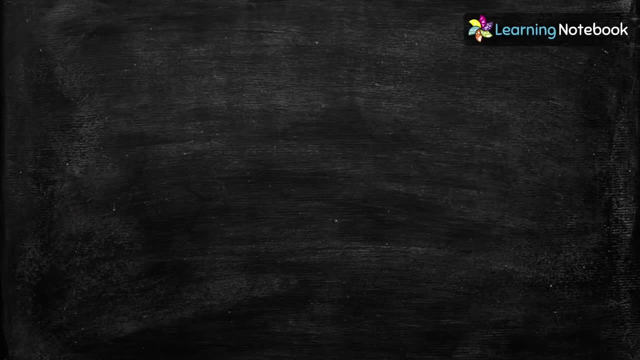 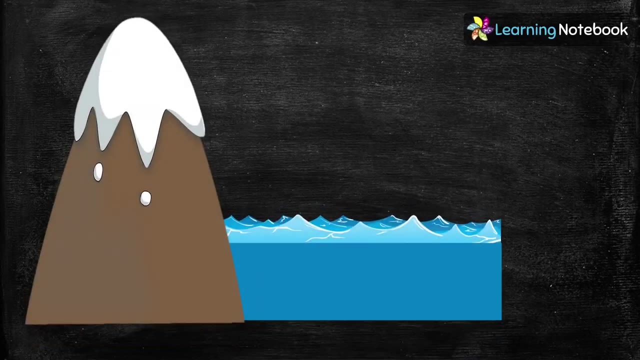 below ground level, we can also express it as negative 4.. Let's take another example: The sea level represents 0. Below the sea level represents negative numbers and above the sea level represents positive numbers. So if we say a place is 0,, we can also express it as negative 0. So if we say a place is 0,, we can also. 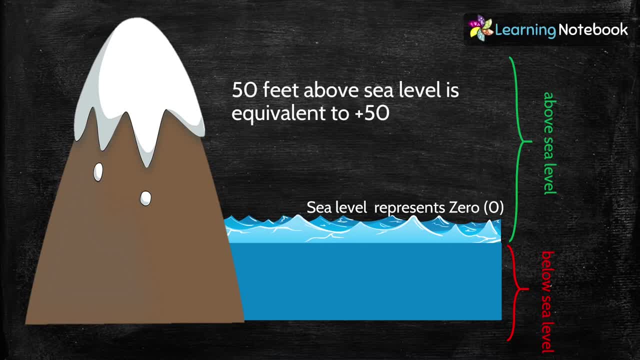 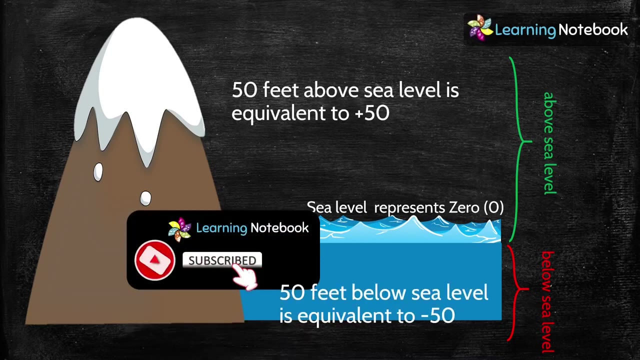 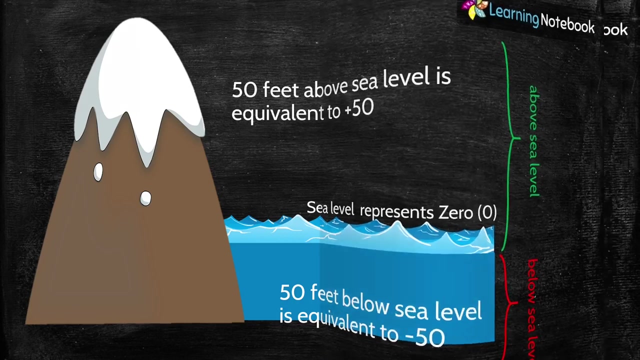 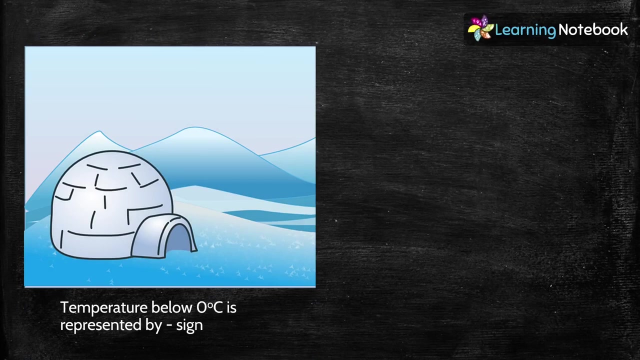 say a place is 50 feet above sea level, that means it is equivalent to positive 50. And if we say 50 feet below sea level, it is equivalent to negative 50.. Similarly, temperature below 0 degrees Celsius is represented by negative sign. For example, temperature in. 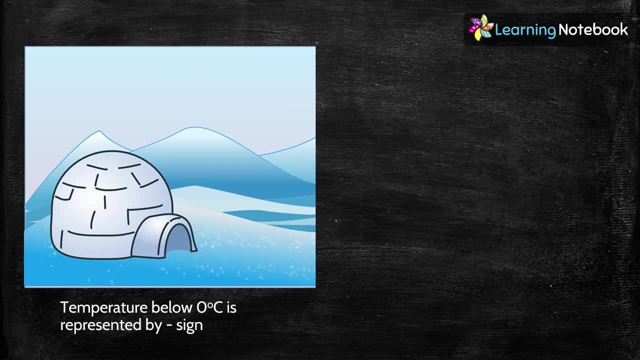 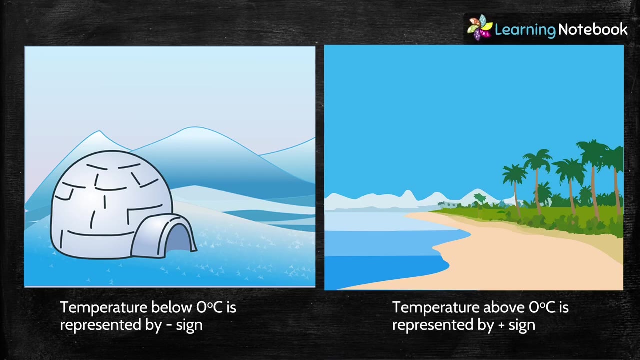 hill stations is written as negative 5 degrees Celsius, negative 10 degrees Celsius, and so on. Also, temperature above 0 degrees Celsius is represented by positive sign. So if we say 0. Below the sea level represents negative 5 degrees Celsius, negative 7 degrees Celsius. 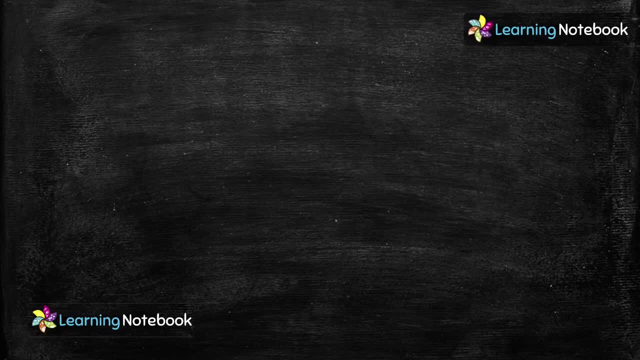 and so on. So we can also say a place is 1 meter above the sea level represents negative 90. And if we say 10 feet above the sea level represents negative 1. So the next symbol for size of a place is negative 20.. So, generally speaking, the given size of a place is equal to 0. That's why the all we describe are their length. Friends do not necessarily mean height. sk excitedly, but I would recommend a mouse being 1 meter tall. So what are the two signs, The two Appearing? 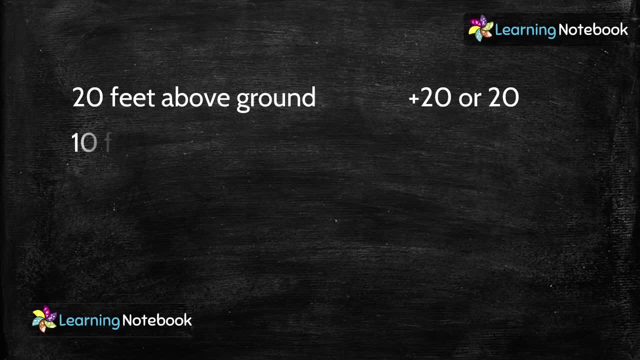 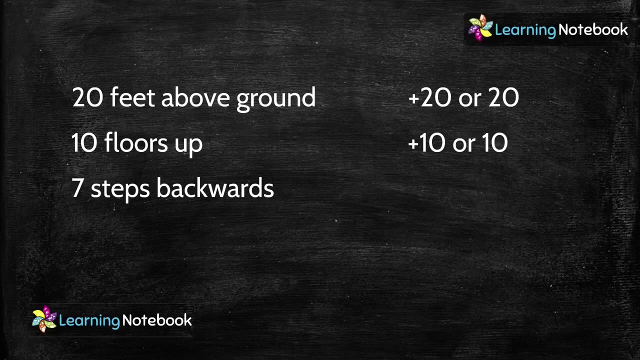 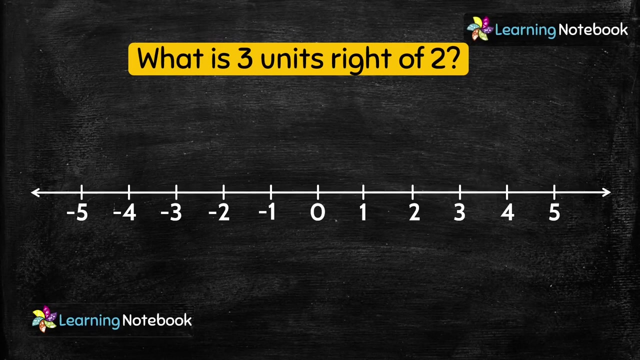 Or only 20.. 10 flows up can be expressed as positive 10 or only 10.. 7 steps backwards: It can be expressed as negative 7. And decrease of 9 points is equivalent to negative 9.. Students, let us once again observe the integers which we represented on the number line. 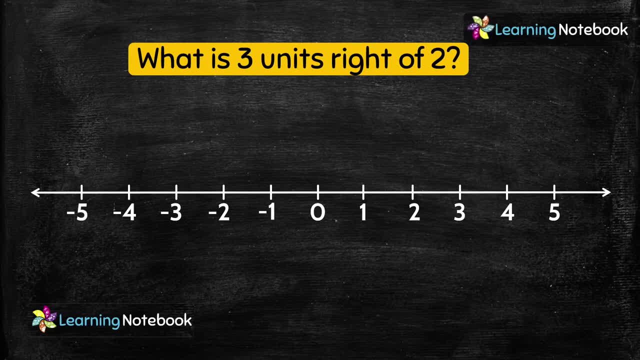 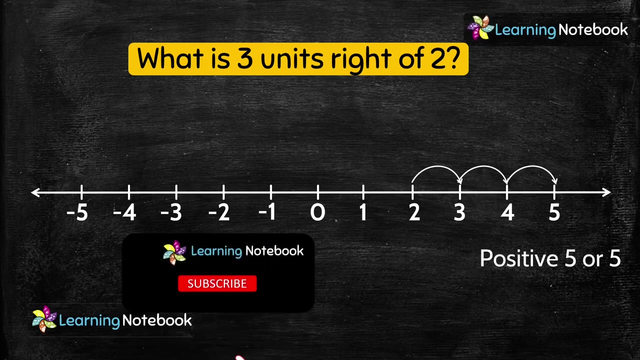 Take a look at integer 2.. 2. If I ask you a question, what is 3 units right of 2?? It means we need to move 3 units or 3 times to the right of number 2.. So we have reached number 5.. 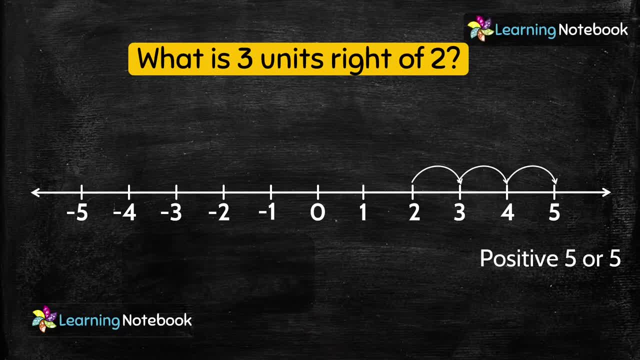 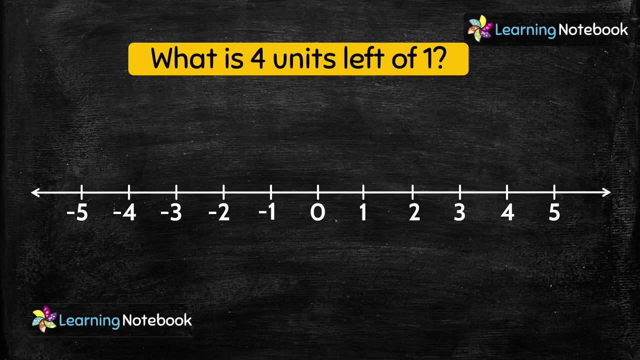 It means 3 units right of 2.. 2 is positive, 5 or only 5.. Similarly, let us take a look at integer 1.. Now if I ask you, what is 4 units left of 1?? It means we need to move 4 units, or 4 times. 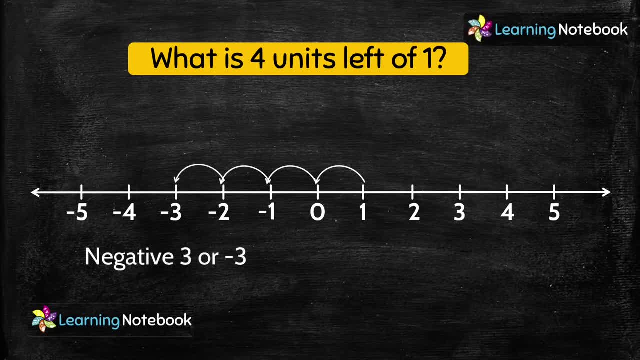 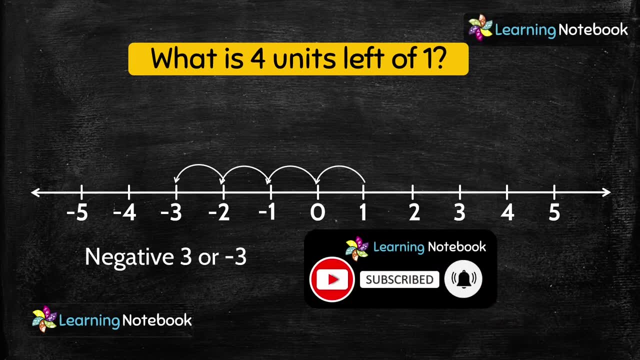 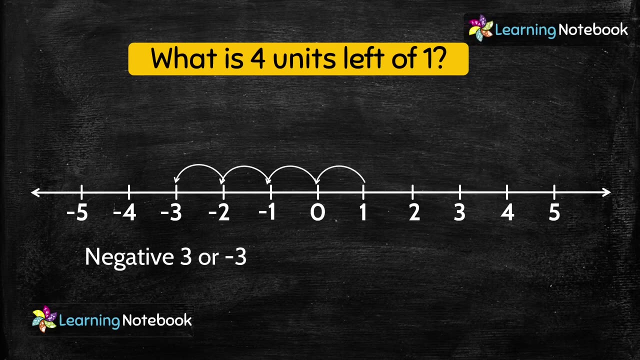 To the left of number 1.. So we have reached negative 3.. It means 4 units left of 1 is negative 3.. So, students, now we know how to represent integers on number line And how to move left or right on number line. 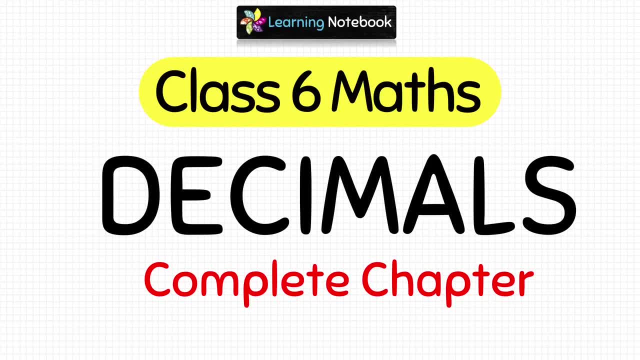 Students. we also have a separate video on complete chapter of decimals for class 6.. In this video, you can learn about place value of decimal numbers, how to represent decimals on number line, how to convert fractions to decimals and decimals to fraction, how to 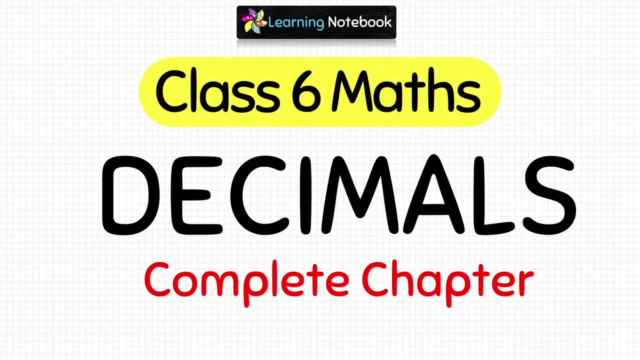 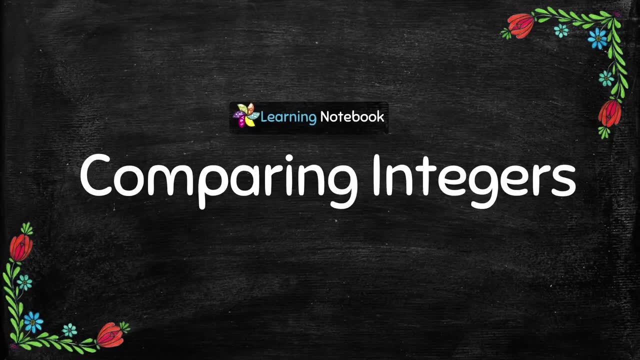 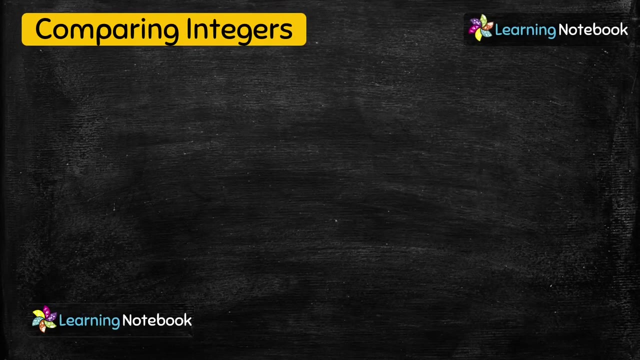 compare and order decimals, addition and subtraction of decimals, and lot more. So I would recommend you to watch this video. You will find its link below in the description box. Now let's continue and learn how to compare integers. To compare integers, we need to understand that the numbers to the right of 0 get bigger. 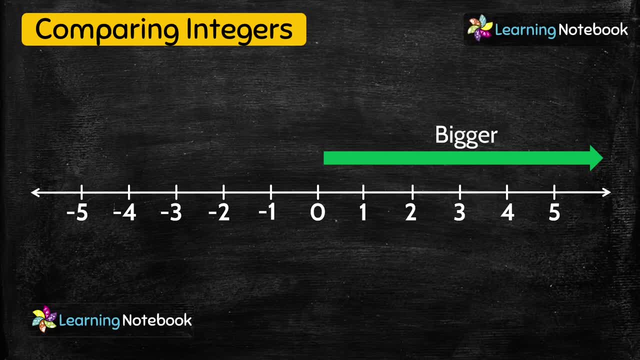 and bigger, While the numbers to the right of 0 get bigger and bigger. So we need to understand that the numbers to the right of 0 get bigger and bigger. So we need to understand that the numbers to the left of 0 get bigger and bigger. 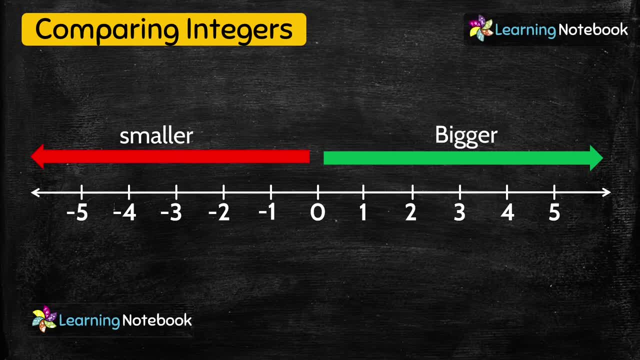 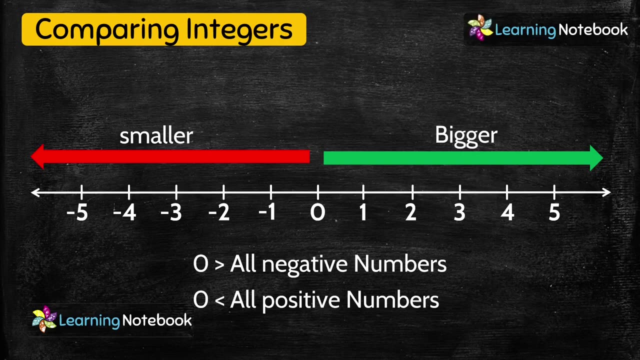 So we need to understand that the numbers to the left of 0 get bigger and bigger. Therefore, 0 is greater than all negative numbers, but 0 is less than all positive numbers. Let's take an example. Let's compare integers to decimals. 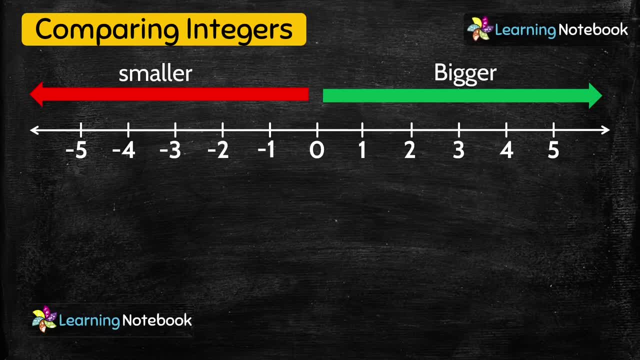 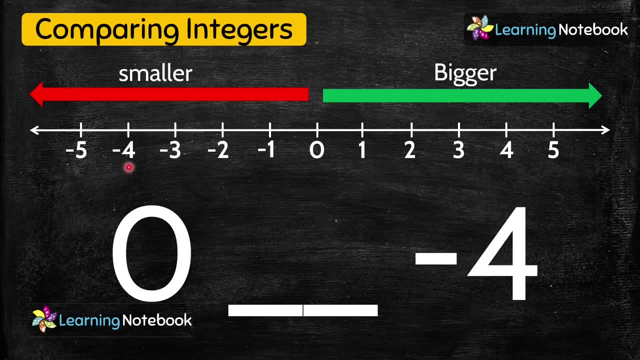 Let's compare integers to decimals. To compare integers to decimals 0 and negative 4.. Since negative 4 is a negative integer and it is found to the left of number 0, it means 0 is greater than negative 4.. Let's see one more example. 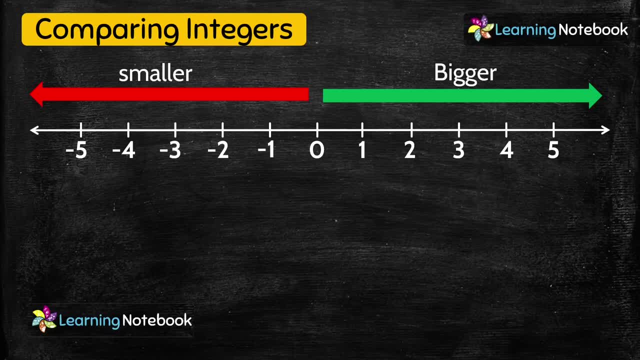 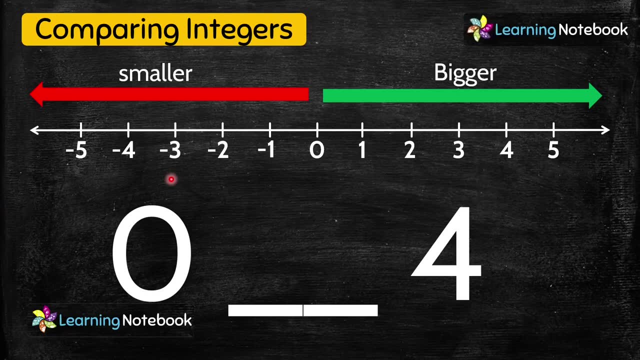 Now let's compare 0 and positive 4.. Now, students, since positive 4 is a positive integer and it is found to the right of number 0,, it means 0 is less than positive 4.. Next to compare integer: 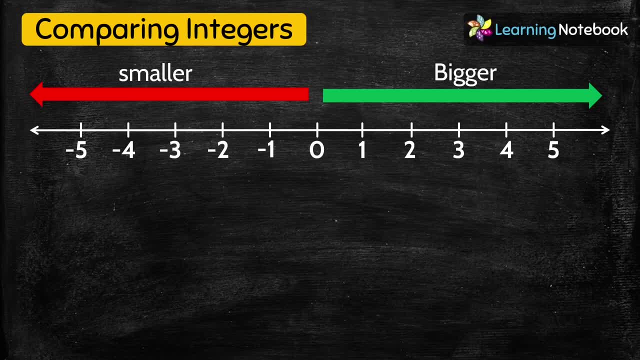 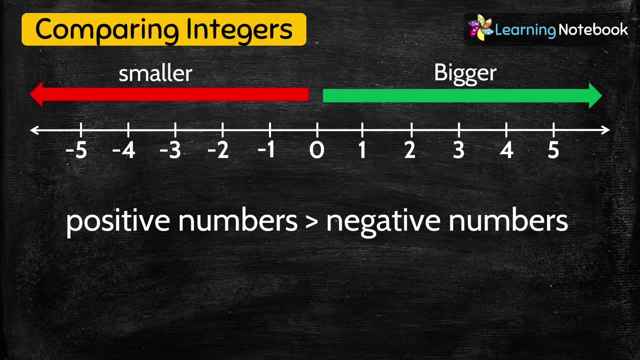 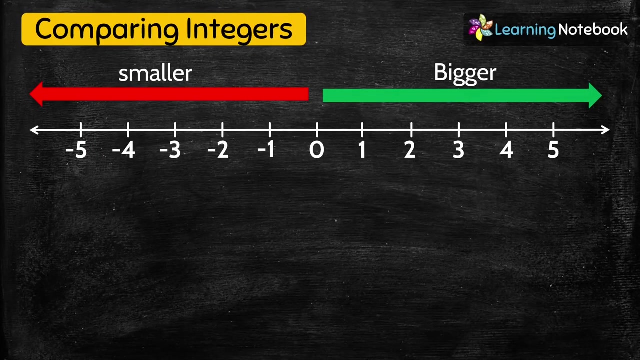 and integer. we also need to understand that all positive numbers are greater than negative numbers. It also means all negative numbers are less than the positive numbers. Let's see an example. Let us compare positive 3 with negative 3.. Let's compare positive 3 with negative 3.. Let's compare positive 3 with negative. 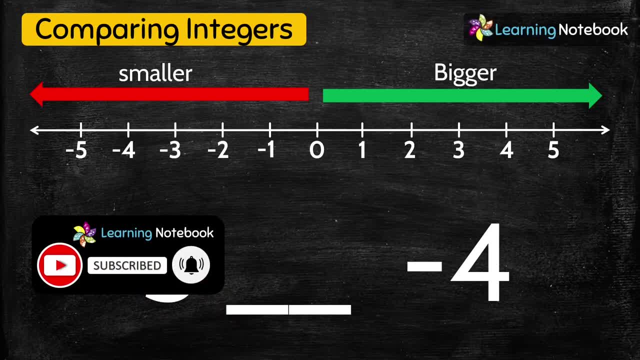 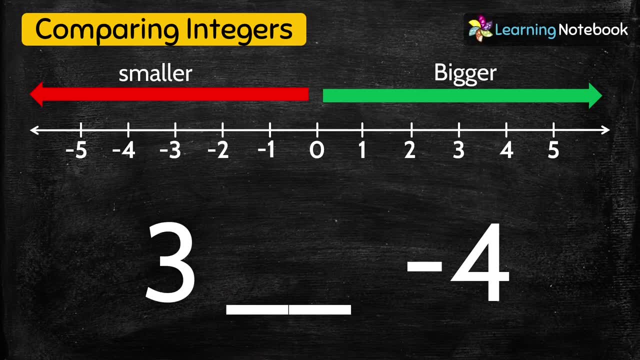 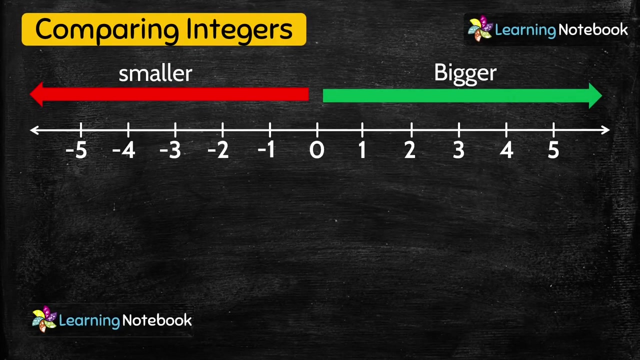 3 and negative 4.. It seems that negative 4 is greater than positive 3. But as we learnt that all positive numbers are greater than the negative numbers, Therefore positive 3 is greater than negative 4.. Now let us compare negative 3 and positive 1. Since we learnt that all negative numbers are less, 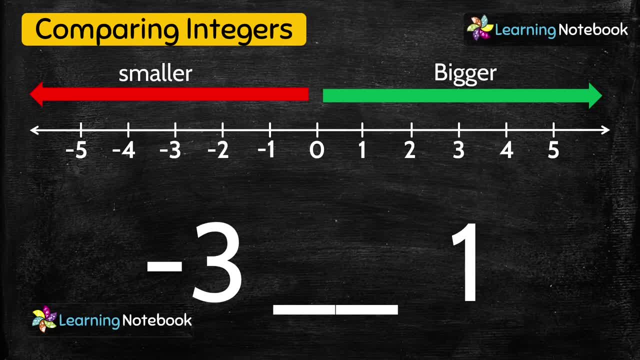 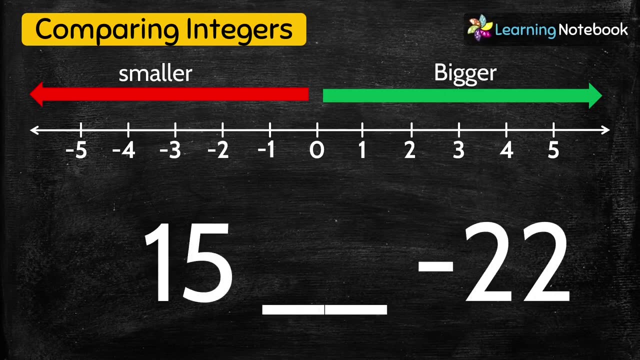 than all positive numbers. Therefore, negative 3 is less than positive 1.. Next let us compare 15 and negative 22.. Again, we know that all positive numbers are greater than all negative numbers. Therefore, 15 is greater than negative 22.. 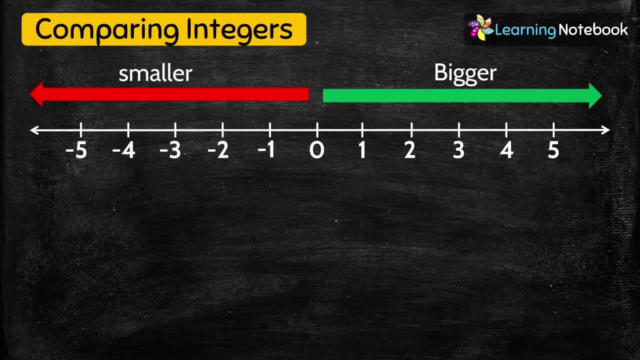 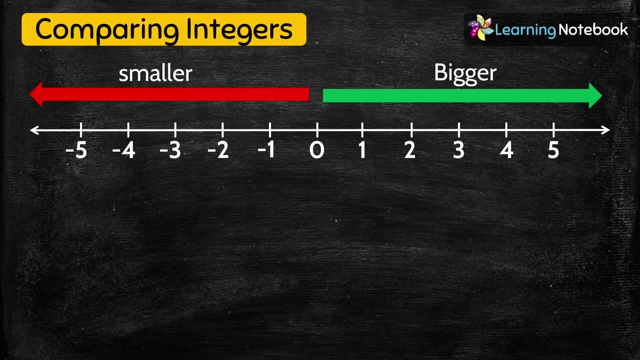 Now what if we compare negative numbers with positive numbers? We learnt that if we move left on the number line, negative number gets smaller and smaller. It means bigger the number, smaller it is. To understand this, let us compare negative 3 and negative 5.. 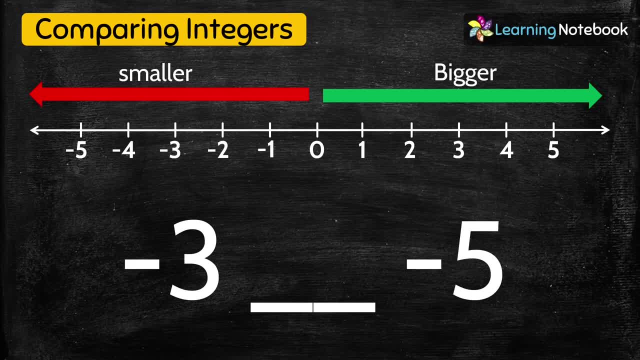 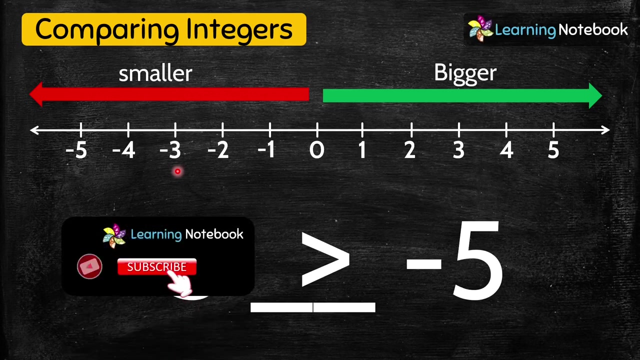 Here it seems that negative 5 is greater than negative 3.. But negative 3 is closer to number 0. So negative 3 must be bigger than negative 5.. If you still not have subscribed to our channel Learning Notebook, then do subscribe it We. 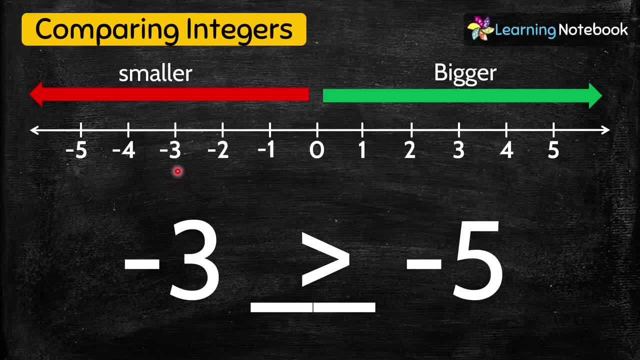 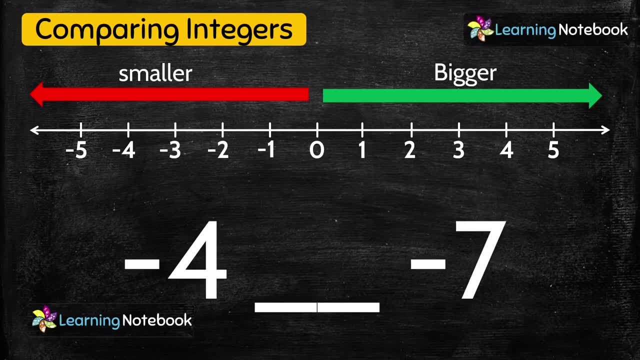 would be very happy if you do, And make sure to press the bell icon. Let's see one more example. Compare negative 4 and negative 7.. Now, since negative 4 is closer to number 0. So negative 4 is greater than negative 7.. 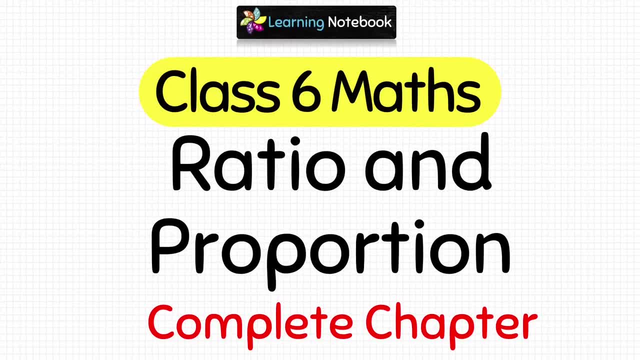 So negative 4 is greater than negative 7.. Students, we also have a separate video on complete chapter of ratio and proportion for class 6.. In this video, you can learn about what is ratio, what is proportion, how to compare ratios. 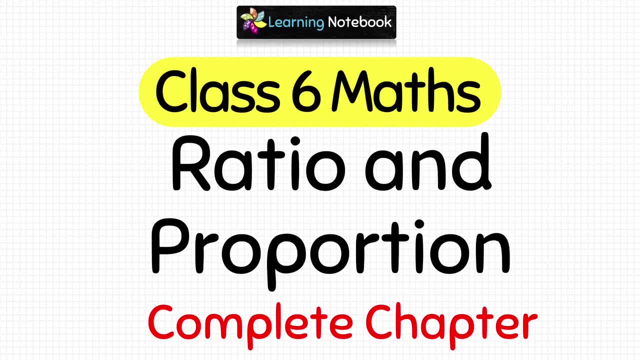 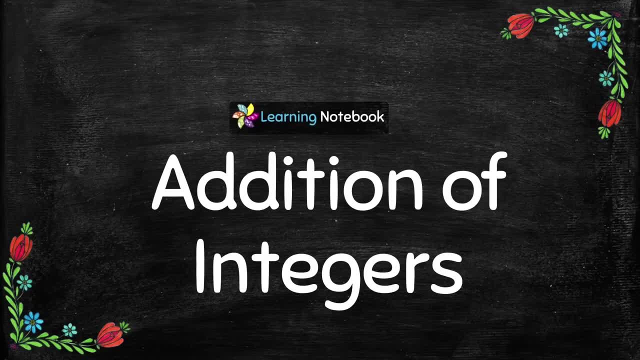 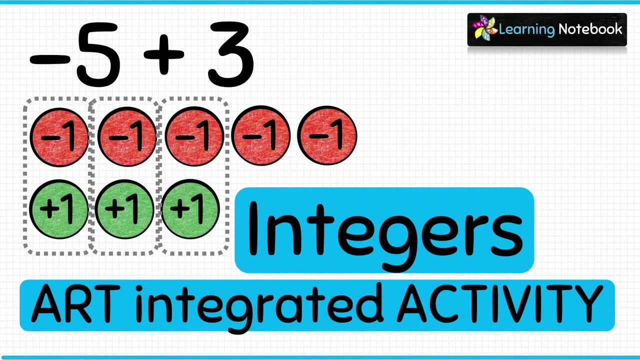 and unitary method. The link to this video is below in the description box. Now let's continue and understand the ratio and proportion of negative 4 and negative 7.. To understand addition and subtraction of integers with the help of interesting and colorful activity, you can refer to our separate video. You will find the link to this video below in the description box. 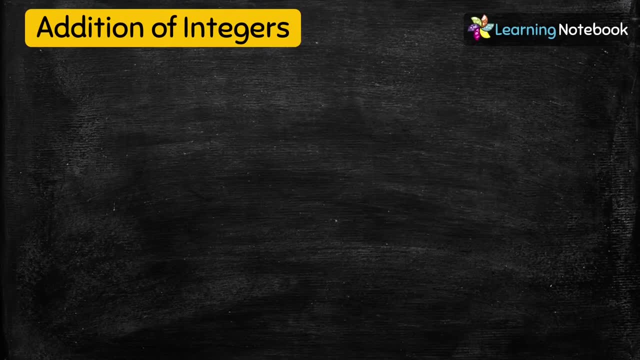 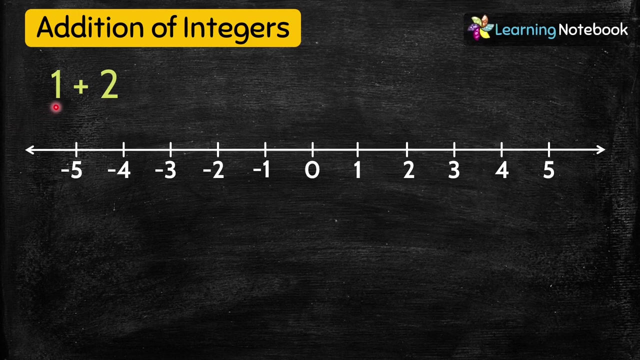 Let's add positive 1 and positive 2.. I know you already know the answer to this, But, students, let me show you how to solve this using number line. Here we have positive 1 and we need to add positive 2.. 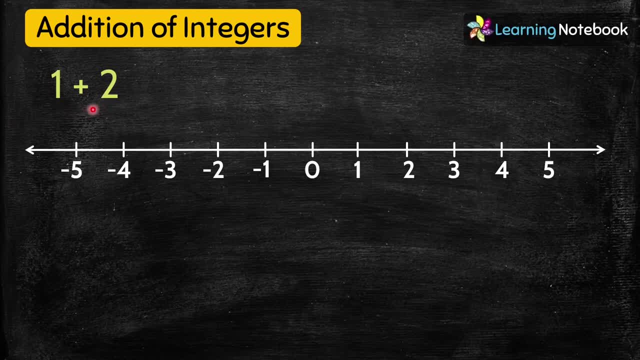 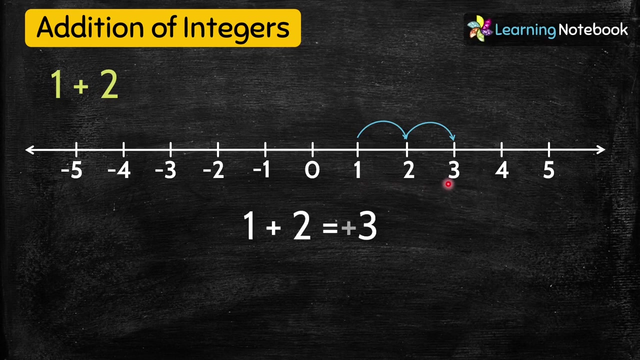 Since 2 is positive, we need to move 2 times, 2 times to the right of 1 on the number line, And thus we have reached 3.. So our answer is positive 3 or 3. It means positive 1 plus positive 2 equals to positive 3.. 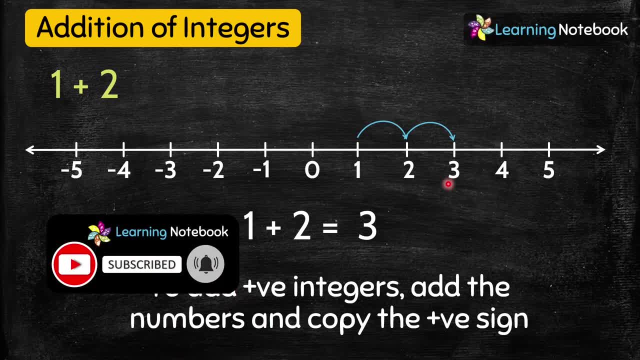 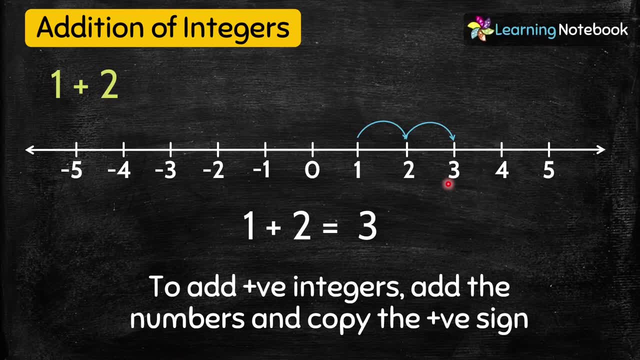 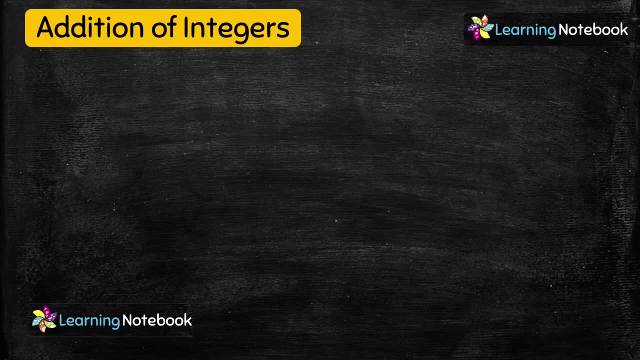 Students. so when we add positive integers, it means positive 2 plus positive 3 equals to positive 3.. So when we add positive integers, we simply add the numbers and copy the positive sign. Let's take another example: Add positive 2 and positive 3.. 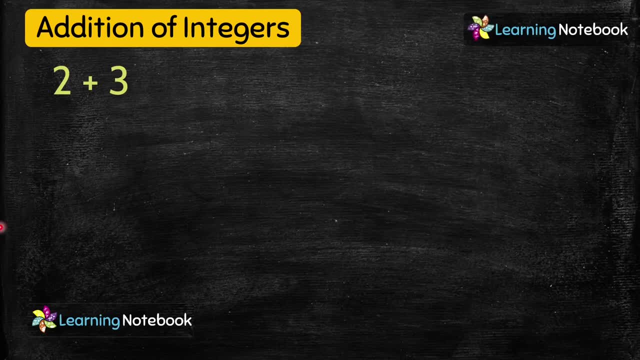 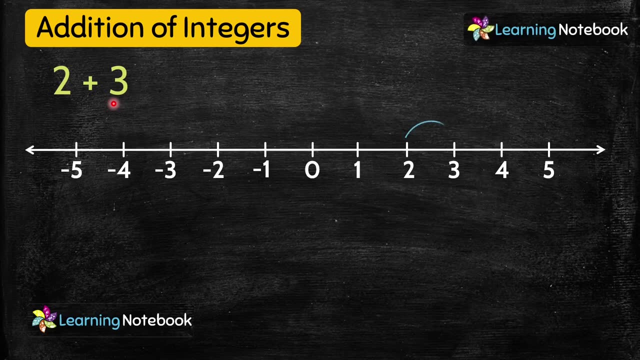 So let's add them using number line. Since 3 is a positive number, we will move 2 times. So we will move 3 times to the right of positive 2.. So we have reached 5.. So it means positive 2 plus positive 3 equals to positive 5 or only 5.. 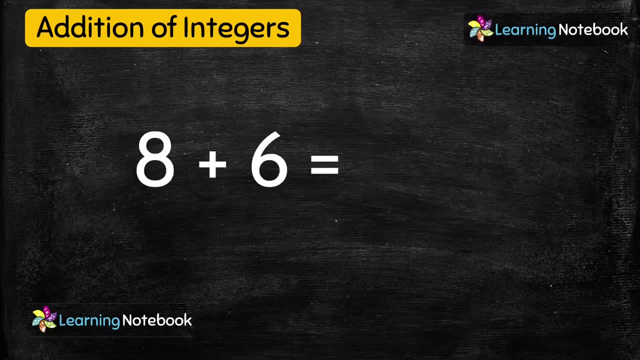 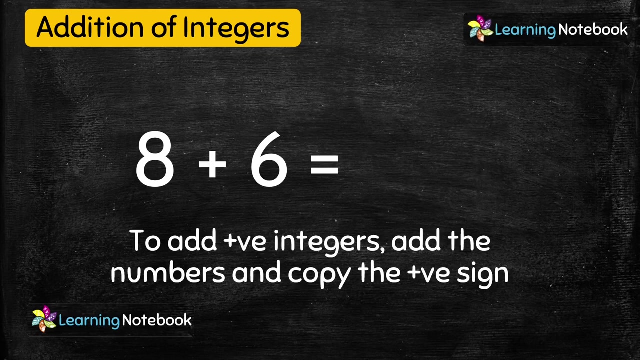 Now let us try another example: 8 plus 6.. Students, we will try to add these integers without number line. Since both are positive numbers, we will simply add them and copy the positive sign. So 8 plus 6 equals to 14.. 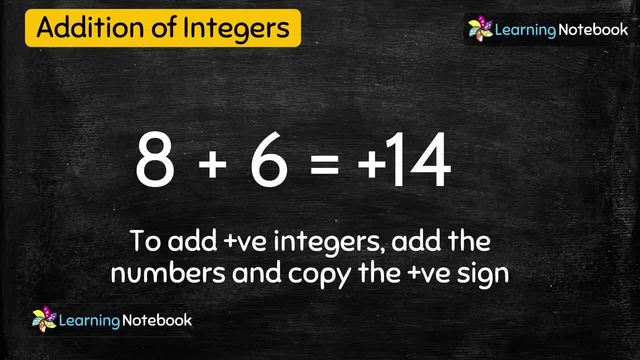 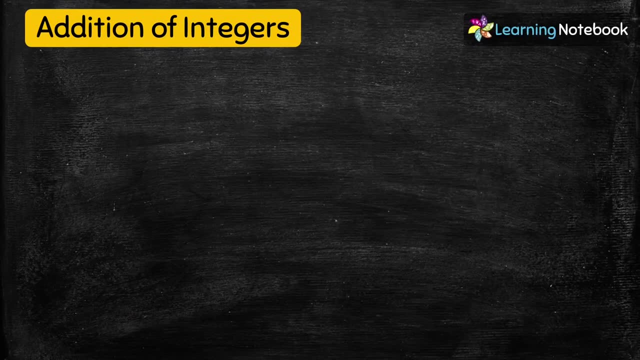 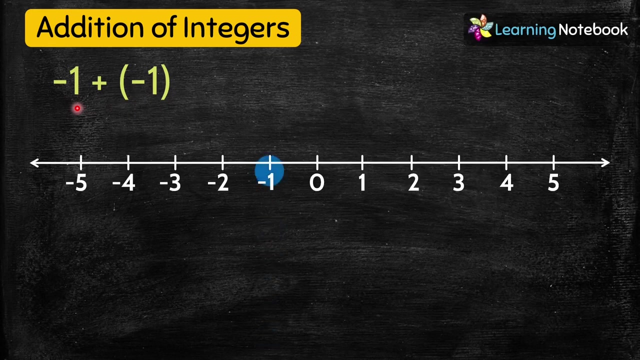 And we will just copy the positive sign. So answer is: 8 plus 6 equals to positive 14 or 14.. Now what if we add two negative integers, For example negative 1 plus negative 1.. So here first number is negative 1.. 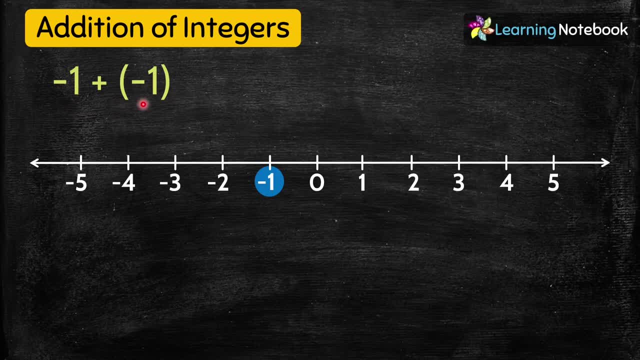 And we are going to add negative 1.. add negative 1 to it, Students, since this is a negative integer. so, instead of moving to the right, we are going to move to the left. So let's move one unit to the left. 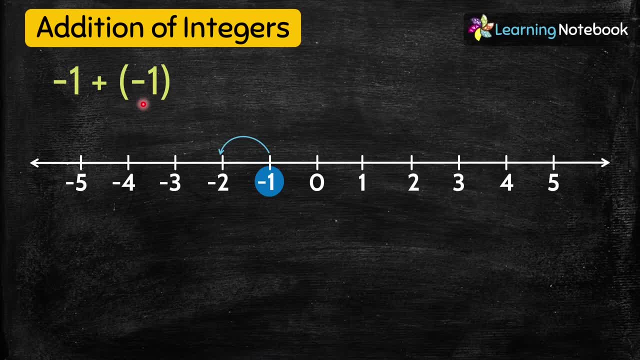 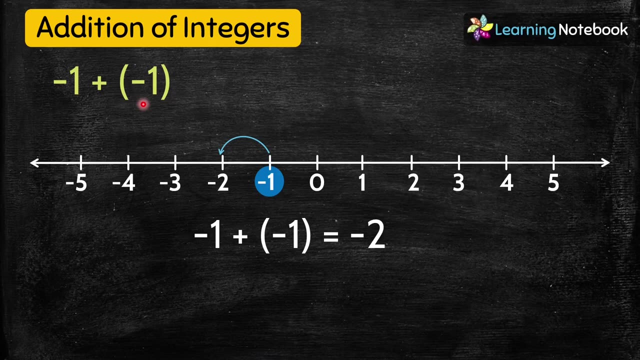 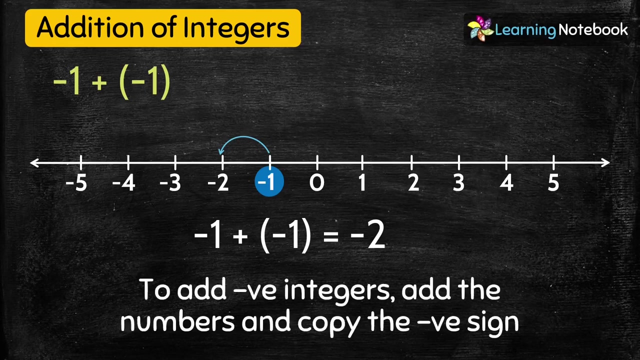 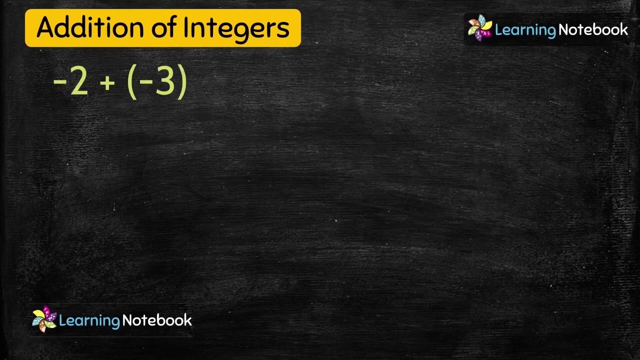 of negative 1. We get negative 2. So it means negative 1 plus negative 1 equals to negative 2. Therefore we observe that to add negative integers, we simply add the numbers and copy the negative. Let's take one more example: Negative 2 plus negative 3. Again, we are adding a negative. 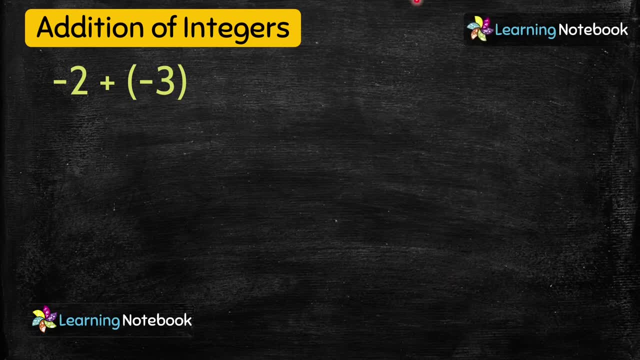 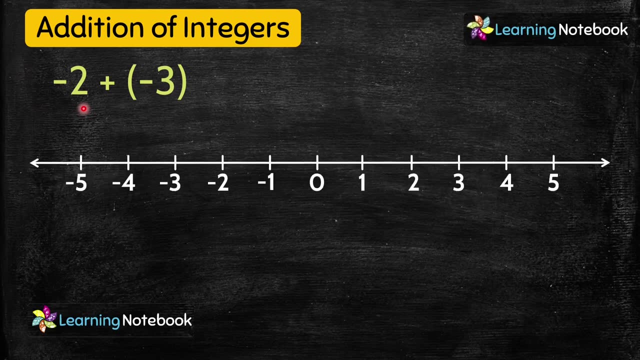 integer to a negative integer. So let's see it on number line. First number is negative 2.. And we are going to add negative 3 to it. So let's move three units to the left of negative 2. We get negative 5. It means negative 2 plus negative 3 equals to negative 5.. 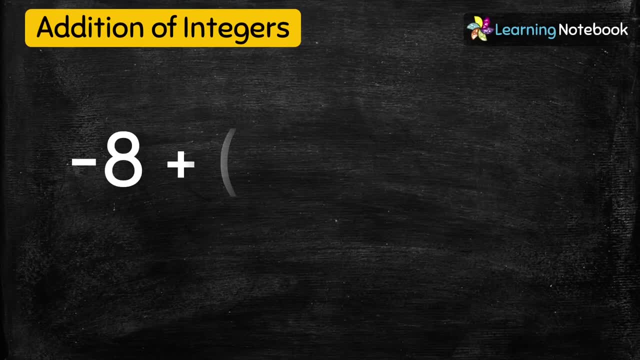 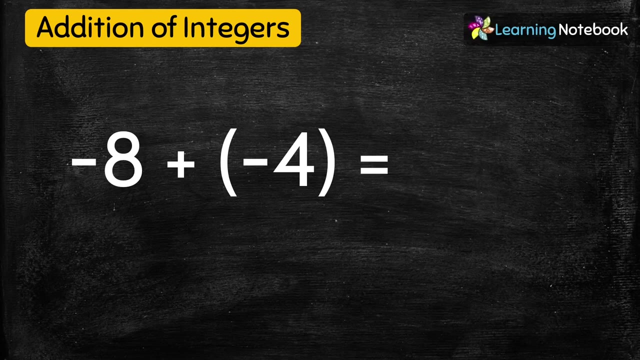 Let's see the next example: Negative 8 plus negative 4.. Students, let us try to add these integers without using number line. Since both of them are negative integers, we will simply add them and copy the negative sign. So 8 plus 4 equals to 12. And we will write the negative sign. So we get the answer as: 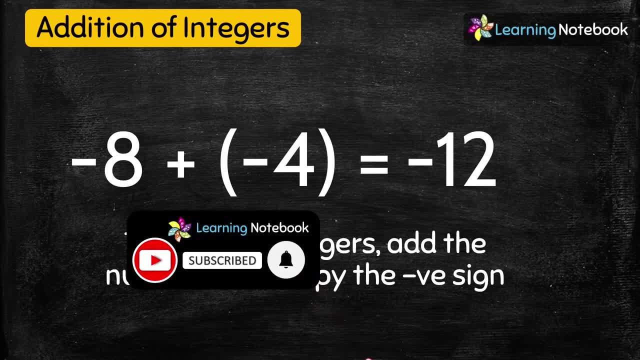 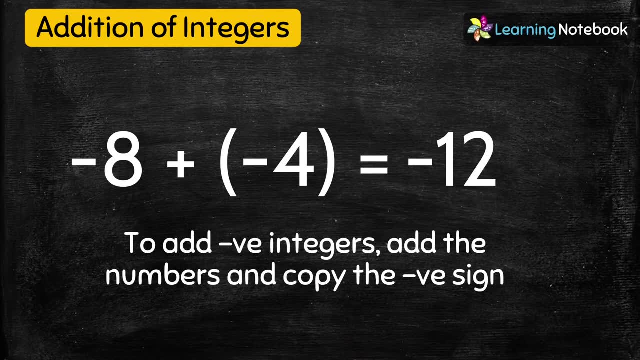 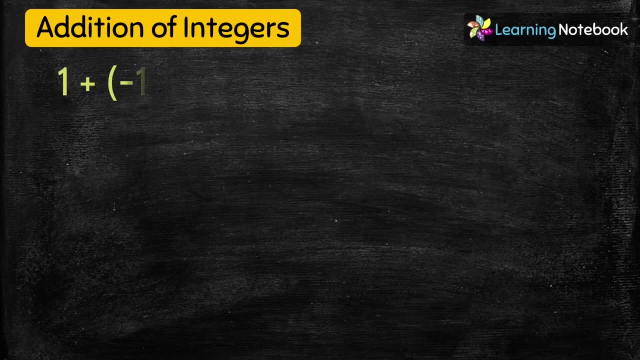 negative 12.. So it means negative 8 plus negative 4 equals to negative 12.. So it means negative 8 plus negative 4 equals to negative 12.. Now, students, let's see how to add positive integers to a negative integer. So let's. 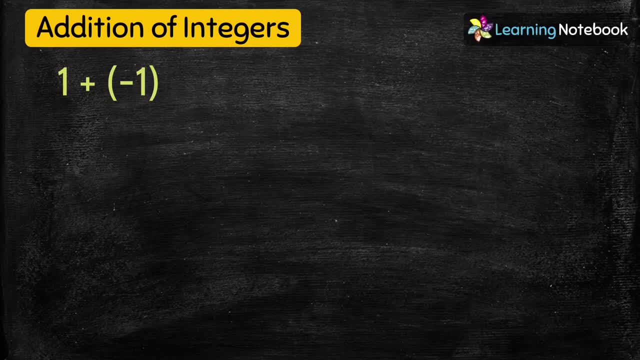 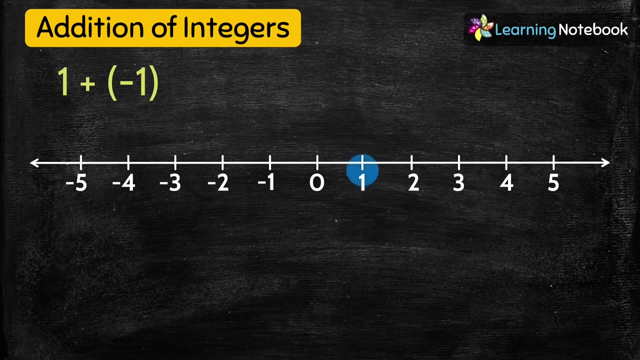 see how to add positive integers to a negative integer. So let's see how to add positive and negative integers. Question is: positive 1 plus negative 1.. So here we are trying to add opposite signs. First number is positive 1 and we are adding negative 1 to 8.. So we 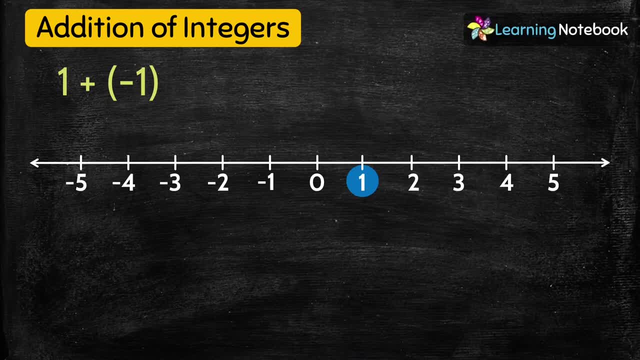 are going to move to the left. So let's move one unit to the left. So let's move one unit to the left. So let's move one unit to the left of positive 1. We get 0. So it means: 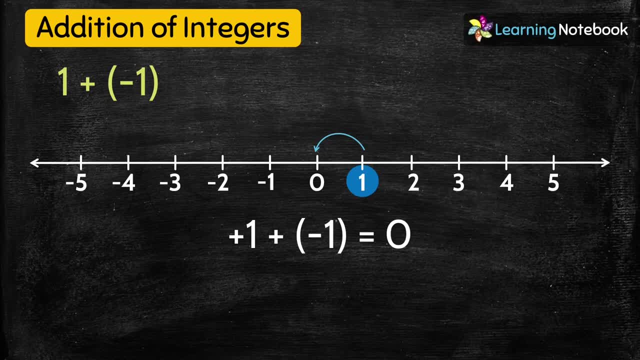 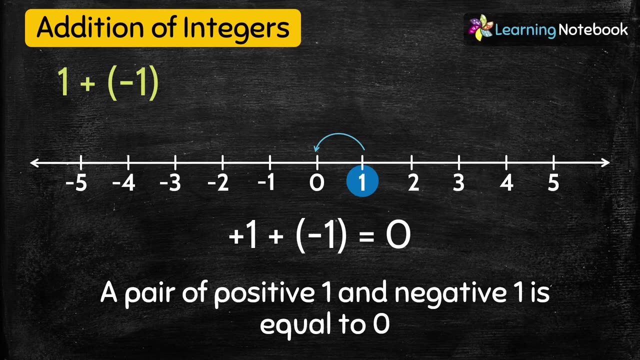 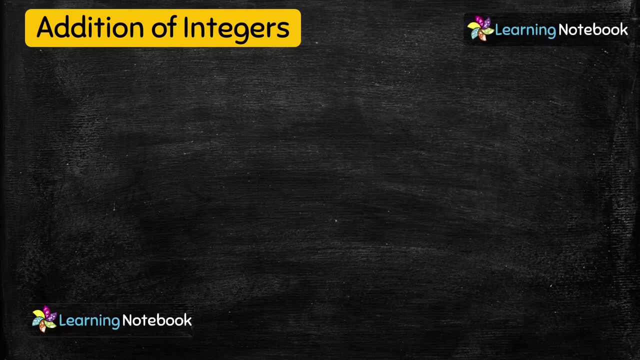 positive 1 plus negative 1 equals to 0.. Students, this is a very important point- that a pair of positive 1 plus negative 1 equals to 0.. So let's move one unit to the left of positive 1 and negative 1 is equal to 0.. Now, students, what if we have to add a positive integer? 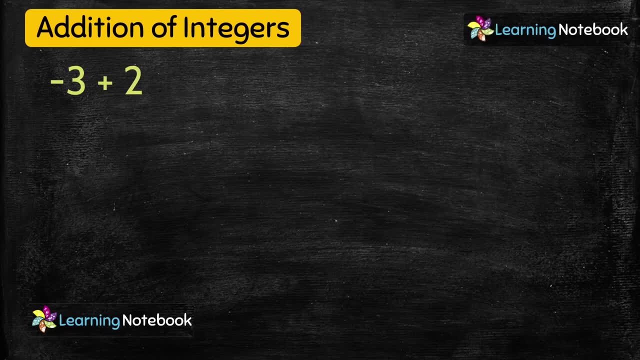 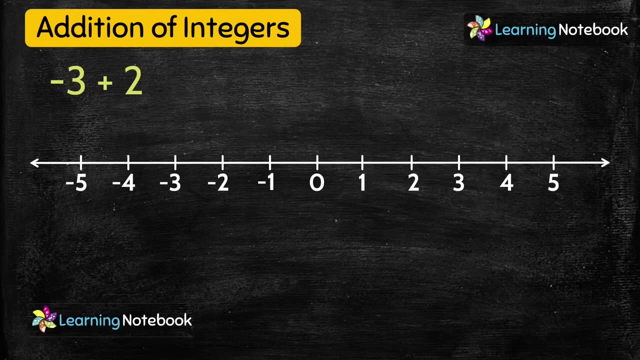 to a negative integer. Let's see such a question: Negative 3 plus positive 2.. So here again we are trying to add opposite signs. So let's move one unit to the left of positive 1 and negative 1 plus negative 1 equals to 0.. Students, let's move one unit to the left of positive 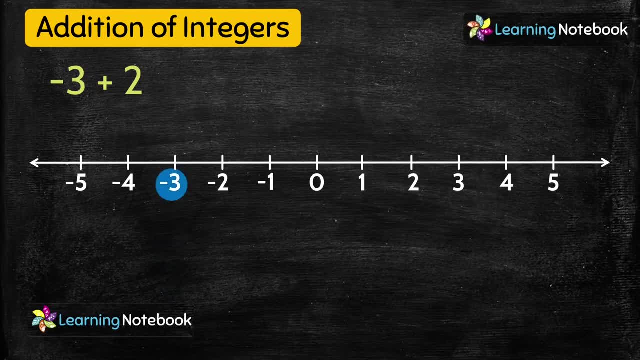 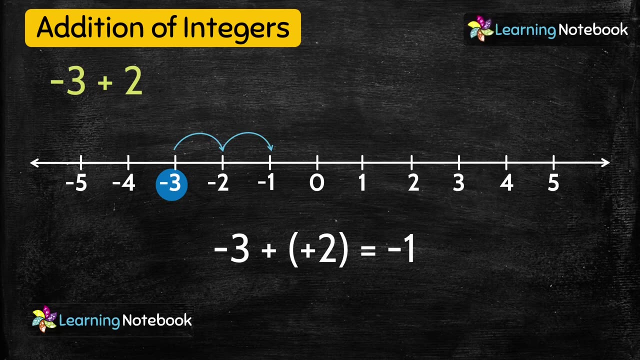 1 and negative 1 equals to 0.. Now, students, we are trying to add opposite signs. First number is negative 3 and we are adding positive 2 to it. So we are going to move to the right. So let's move two units to the right of negative 3.. We get negative 1.. So it means negative. 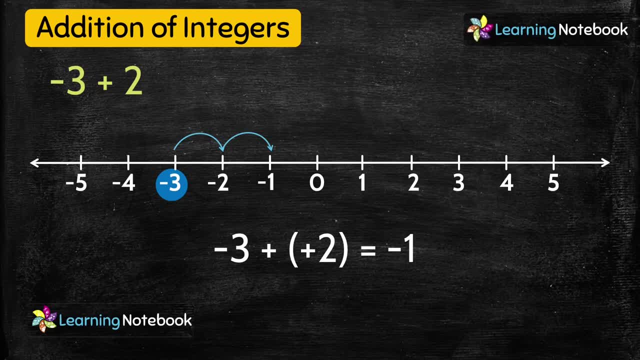 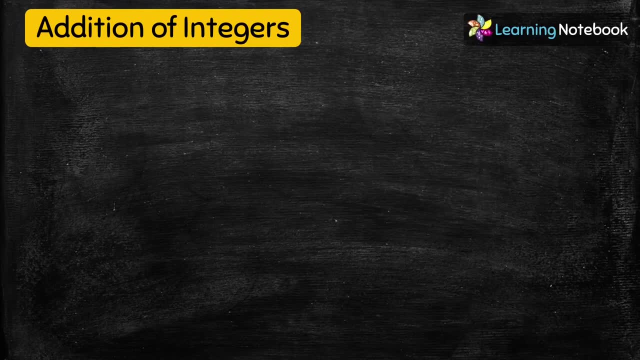 3 plus positive 1 equals to 0.. Students, let's move one unit to the left of positive 2 and 2 equals to negative 1.. Our next question is negative 2 plus positive 7.. So here again we are adding opposite sign. First number is negative 2 and we are adding positive 7. 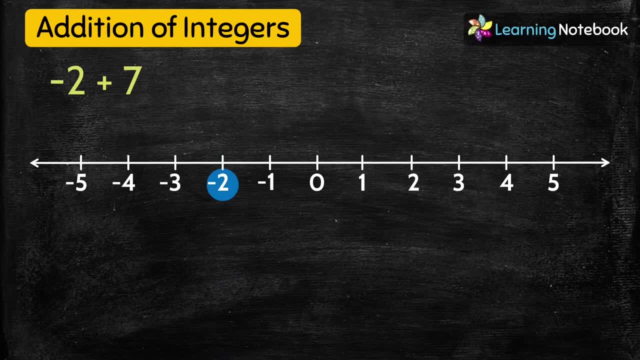 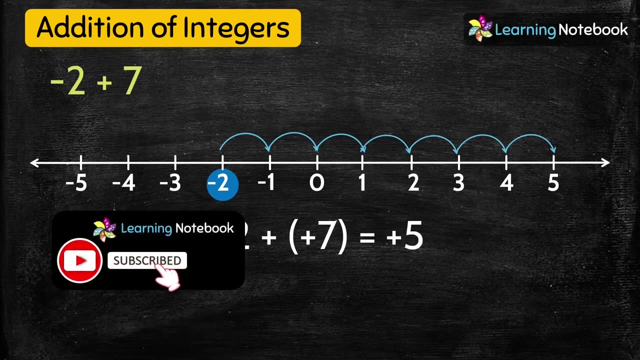 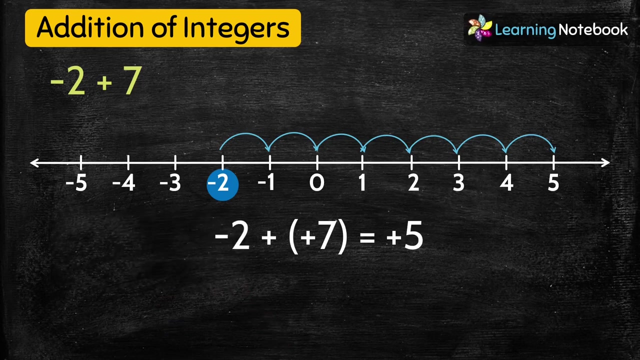 to it. So we will move to the right. Let's move 7 units to the right of negative 2. We get positive 5. So it means negative 2 plus positive 7 equals to positive 5. So, students, we observe. 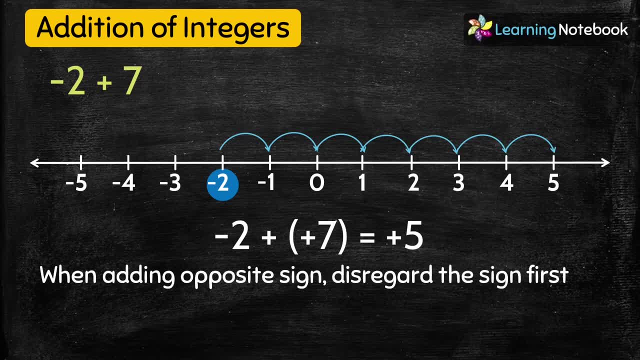 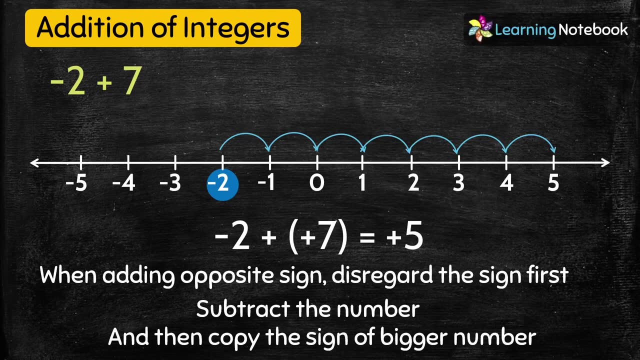 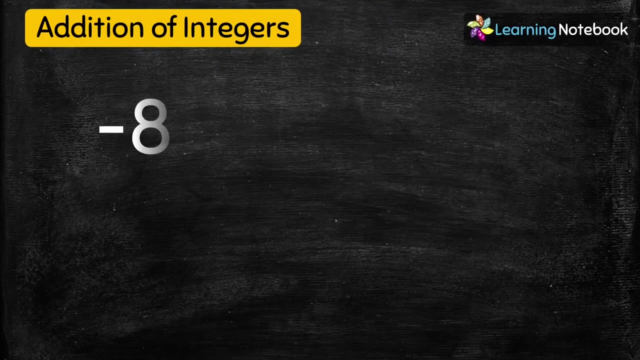 that when we add opposite sign integers, we will disregard the sign first, Then we will subtract the numbers and copy the sign of the bigger number. Let's see the next question: Negative 8 plus positive 5.. Students, let's solve this question. 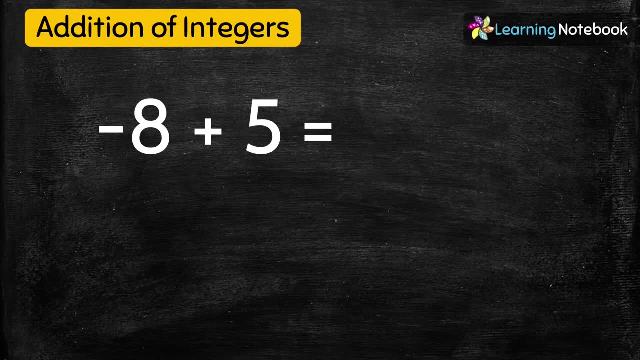 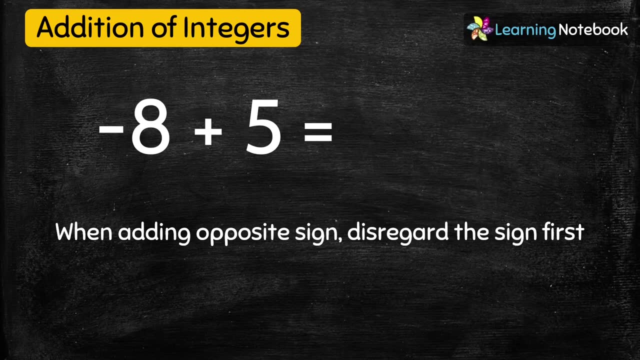 without using number line. So first we can see that these numbers are of opposite sign, So we will disregard their sign. So it means numbers are 8 and 5.. Now let's subtract these numbers: 6, 8, 5.. 8, 5.. 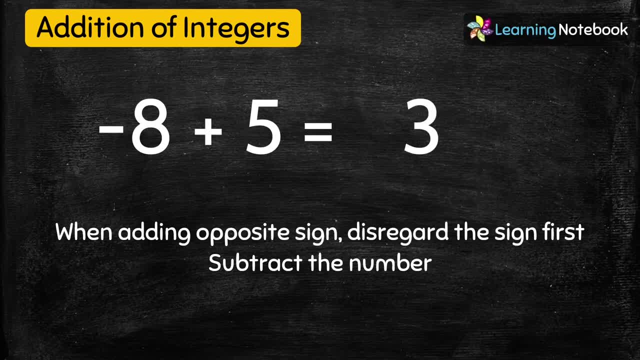 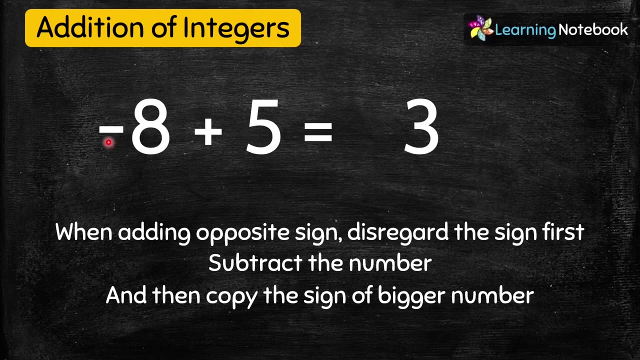 8, 5. Minus 5 equals to 3.. Now we will copy the sign of bigger number Here. bigger number is 8. And it has negative sign to it. So we will put negative sign And we get the answer as negative 3.. 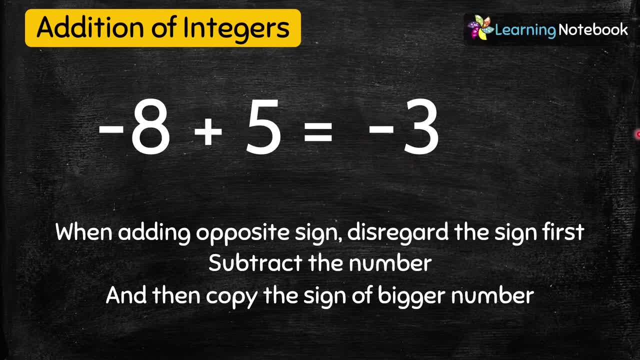 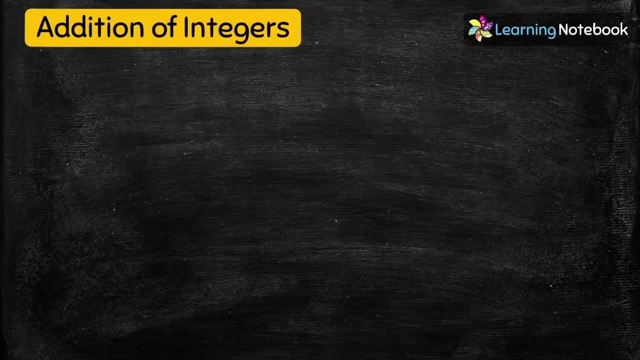 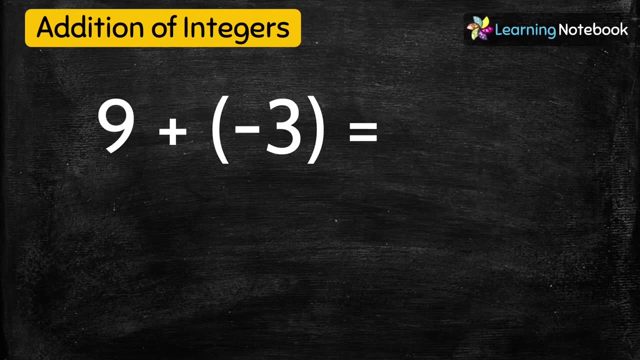 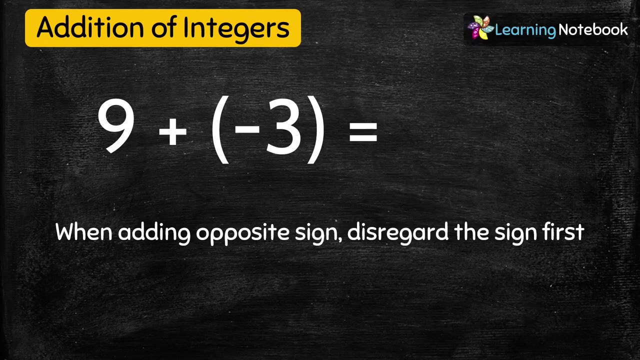 So negative 8 plus positive 5 equals to negative 3.. Let's do one more question: Positive 9 plus negative 3. Again we are adding numbers of opposite sign, So we will disregard their sign. So numbers are 9 and 3.. 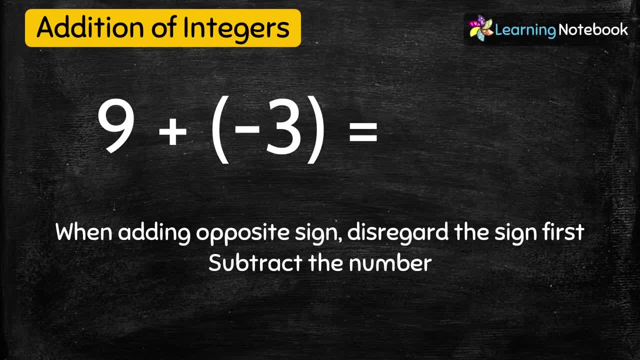 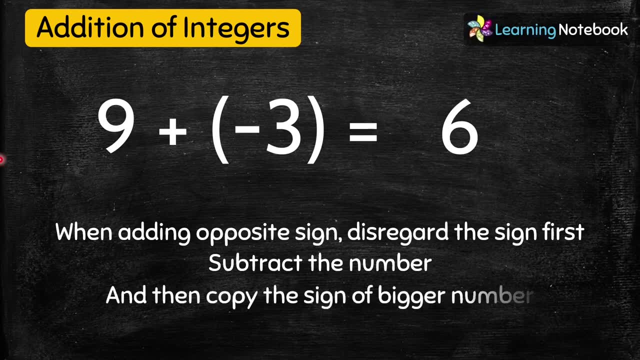 Next we will subtract these numbers: 9 minus 3 equals to 6.. Then we will copy the sign of bigger number Here: bigger number is 9. And it has positive sign to it. So we will put positive sign here. So we get the answer as: 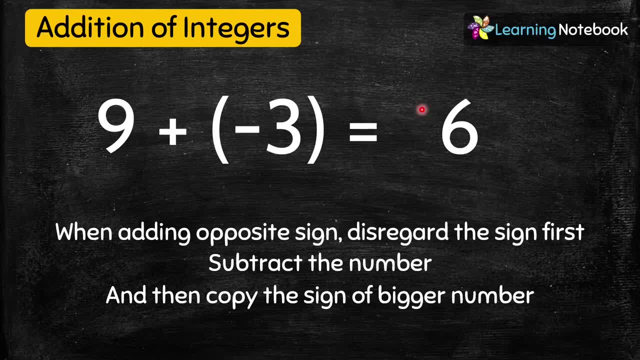 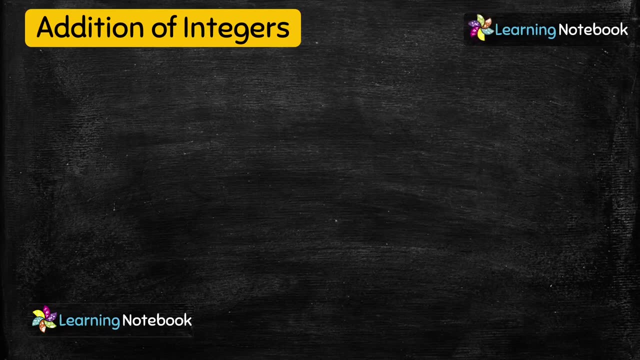 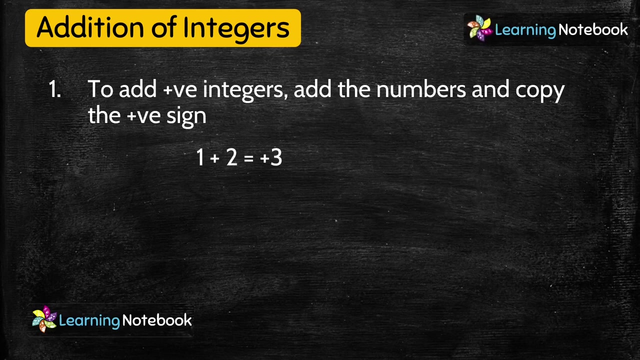 Positive 6 or simply 6.. So 9 plus negative 3 equals to 6.. So let's summarize the rules. to add the integers, To add positive integers, Add the numbers and copy the positive sign. For example, Positive 1 plus positive 2 equals to positive 3.. 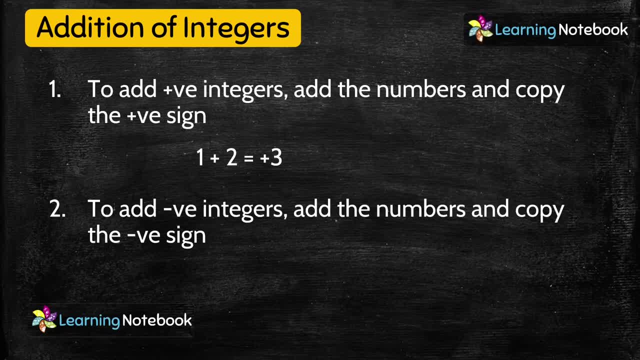 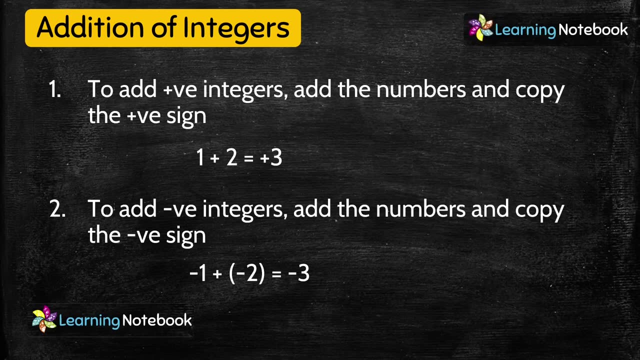 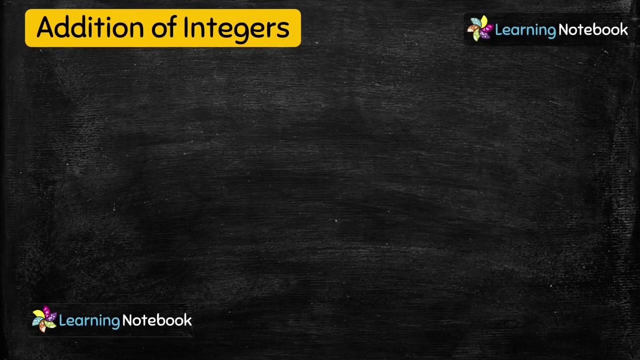 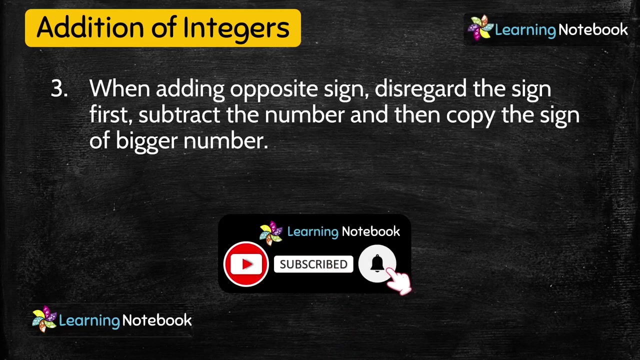 Next rule is To add negative integers. Simply add the numbers and copy the negative sign. For example, Negative 1 plus negative 2 equals to negative 3.. And lastly, When adding opposite sign, Disregard the sign first. 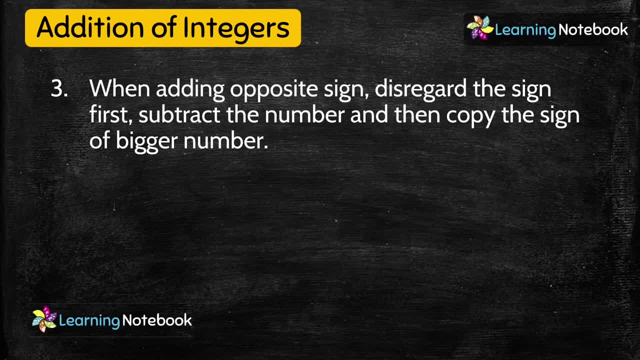 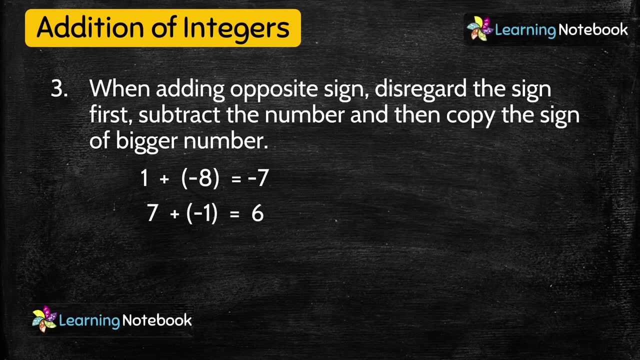 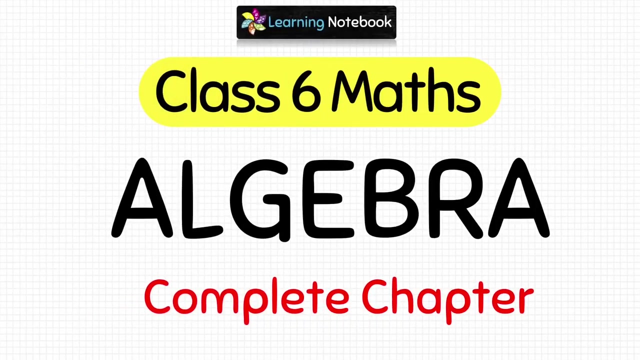 Subtract the number And then Copy the sign of bigger number. For example, 1 plus negative 8 equals to negative 7.. Subtract the number 7 plus negative 1 equals to 6.. Students, we have a separate video on complete chapter of algebra for class 6.. 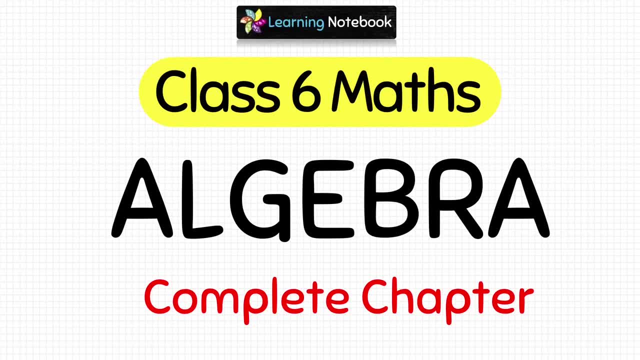 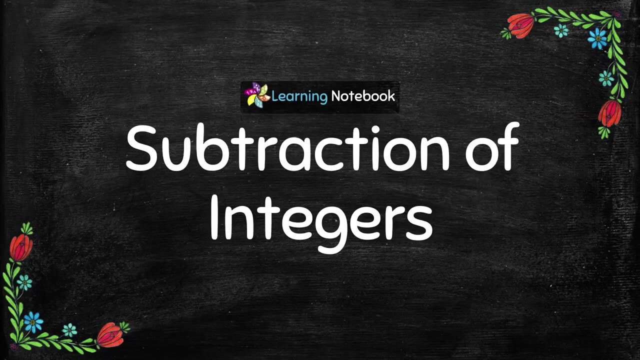 Here you can learn about introduction to algebra. what is algebraic expression, algebraic equation, rules from geometry and arithmetic, and lot more. So I would recommend you to watch this video. You will find its link below in the description box. Now we will understand subtraction of integers. 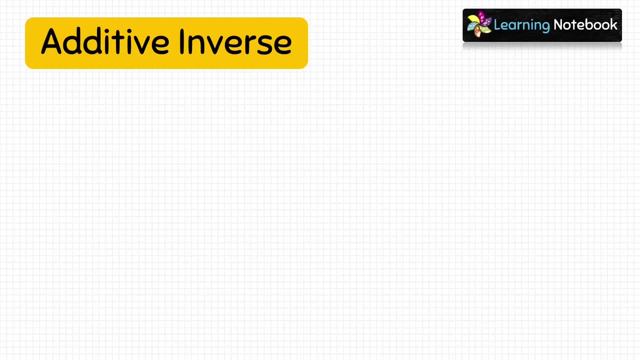 To learn subtraction of integers first we need to understand additive inverse Students. this is a very important concept, So listen carefully. Let's consider the numbers negative 4 and 4, negative 8 and 8, negative 20 and 20.. 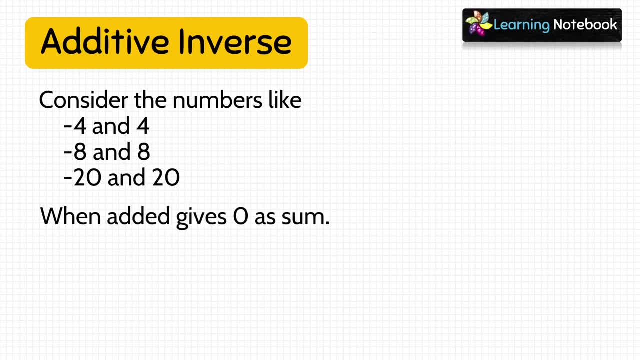 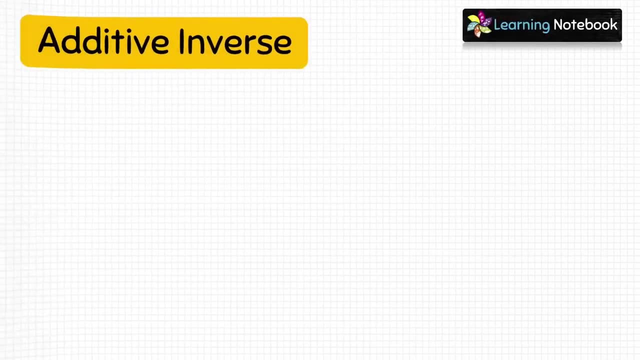 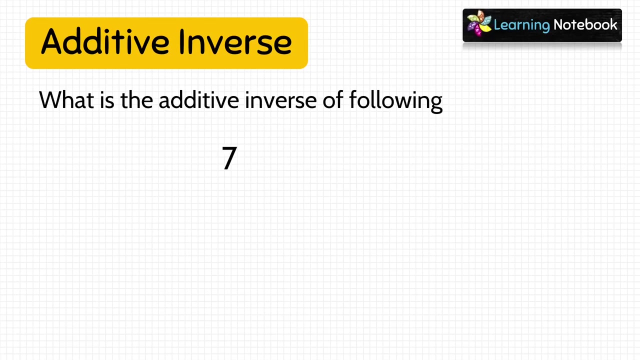 When such numbers are added, they give the sum as 0. So, students, such integers are called additive inverse of each other. So can you tell me what is the additive inverse of 7?? Yes, it is negative 7.. 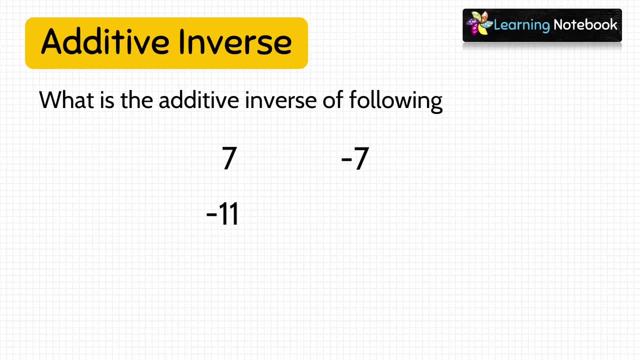 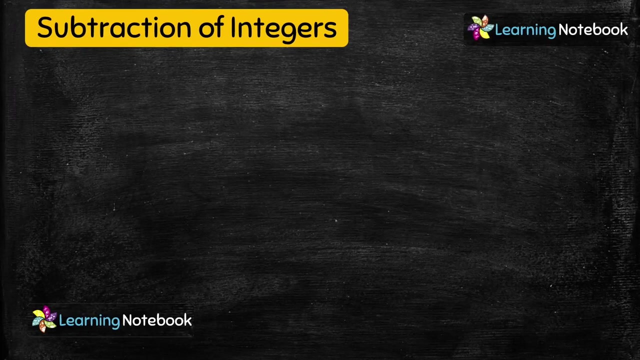 Additive inverse of negative 11 is 11.. And similarly, additive inverse of negative 10 is 10.. So now we are going to use this concept of additive inverse to subtract the integers. Let's do a question: 2 minus 1.. 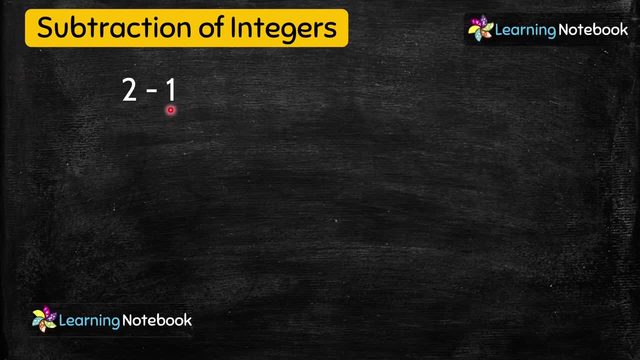 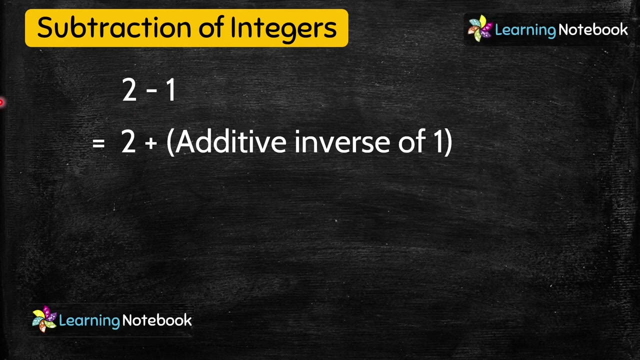 So here we are subtracting positive 1 from positive 2.. Students, to subtract an integer from another integer, it is enough to add the additive inverse of the integer that is being subtracted. So here 2 minus 1 equals to 2 plus additive inverse of 1.. 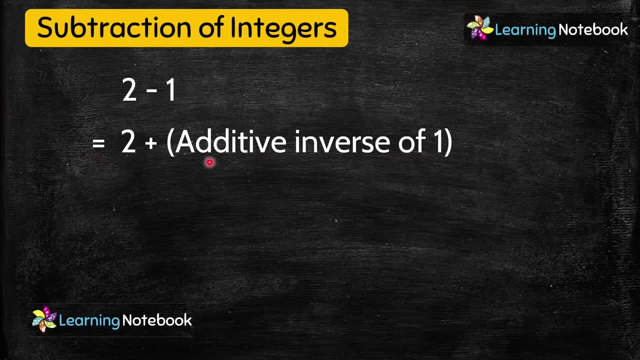 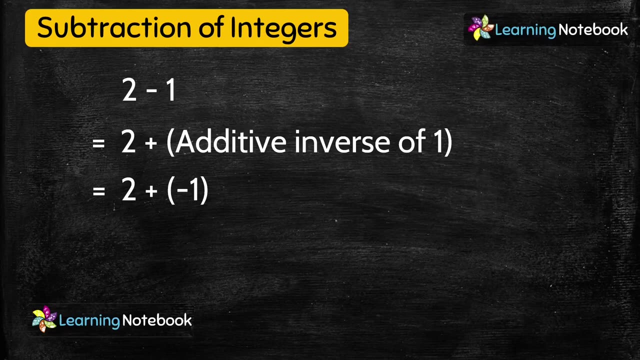 And what is additive inverse of 1?? It is negative 1. Negative 1.. Therefore, 2 minus 1 equals to 2 plus negative 1. Now we can apply the rule of addition. Here we are adding opposite signs, So disregard the sign of the numbers and subtract them. 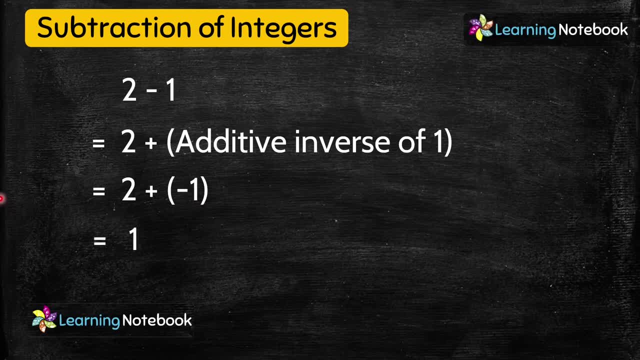 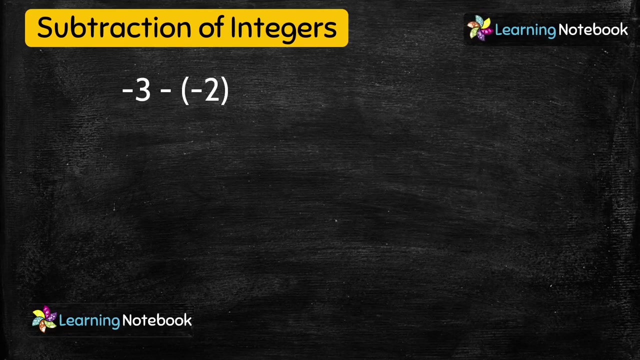 2 minus 1 equals to 1, And then we will put the sign of the bigger number, 2, Which is positive. So answer is positive 1. So it means 2 minus 1 equals to positive 1 or simply 1. Now let's subtract two negative integers. 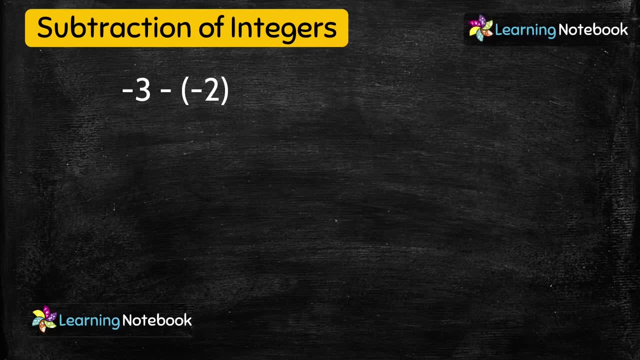 Question is: 2 minus 1 equals to 2 plus negative 1, Negative 3 minus negative 2. So here we are, subtracting negative 2 from negative 3. To subtract these two integers It is enough to add additive inverse of negative 2. 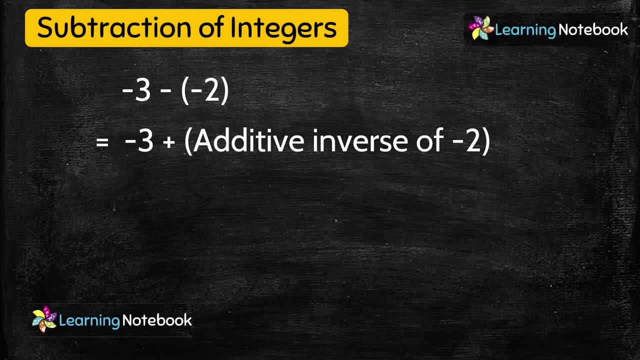 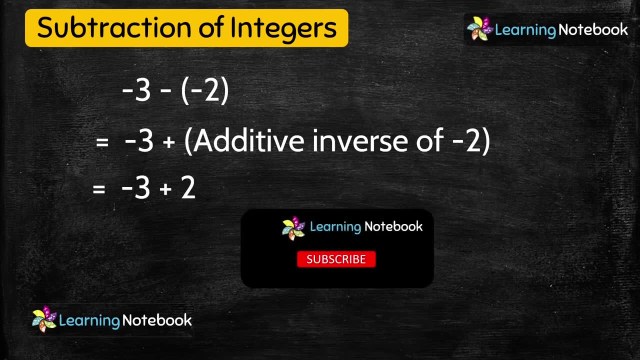 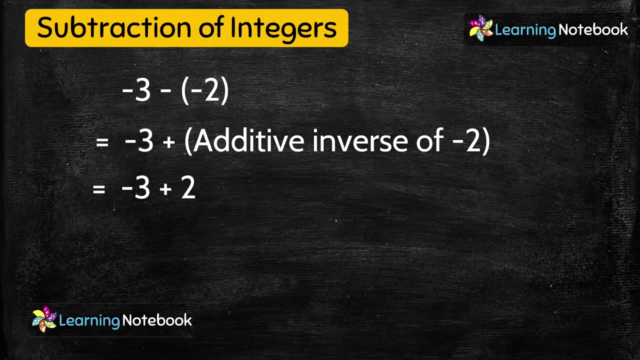 So we get negative 3 plus additive inverse of negative 2, And additive inverse of negative 2 is positive 2, So we get negative 3 plus 2. Now let's add them, Disregard the sign and subtract the numbers, So 3 minus 2 equals to 1. 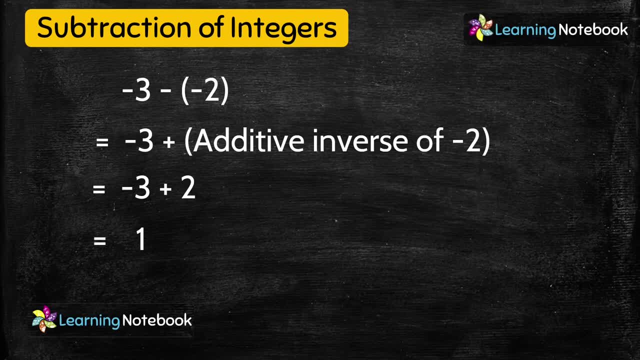 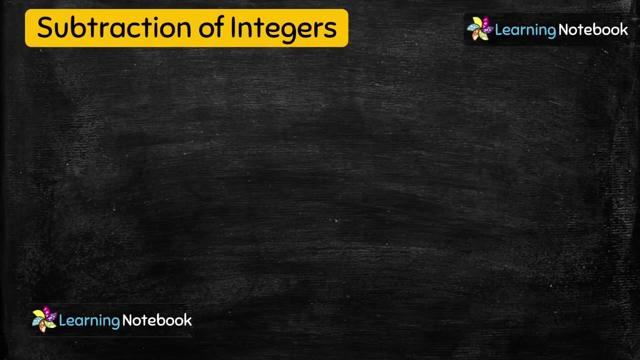 And then we will put the sign of the bigger number, 2, The sign of the bigger number, which is 3, And its sign is negative. So our answer is negative: 1. Now let's subtract one negative integer and one positive integer. Question is Negative 1 minus positive 4. 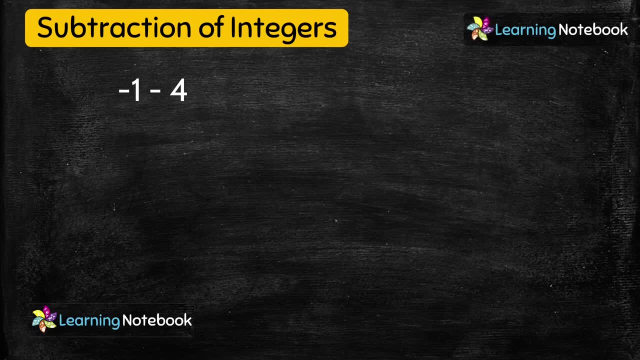 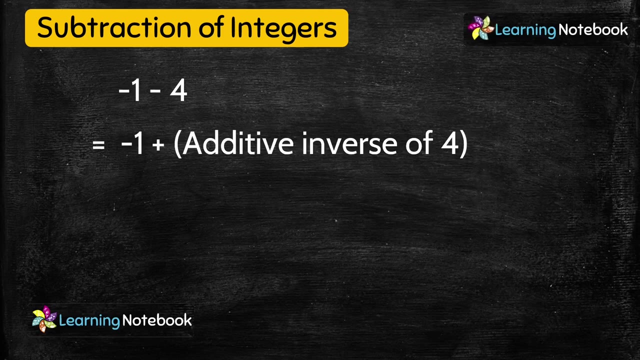 So here we are subtracting 4 from negative 1. Again, students, To subtract these two integers, It is enough to add additive inverse of 4, And additive inverse of 4 is negative 4. So now we will add these two integers, Since both of them are negative integers. 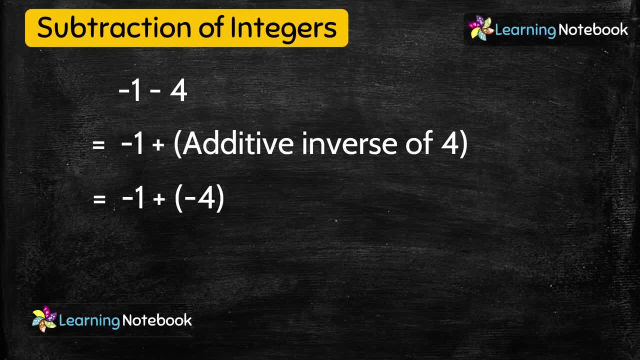 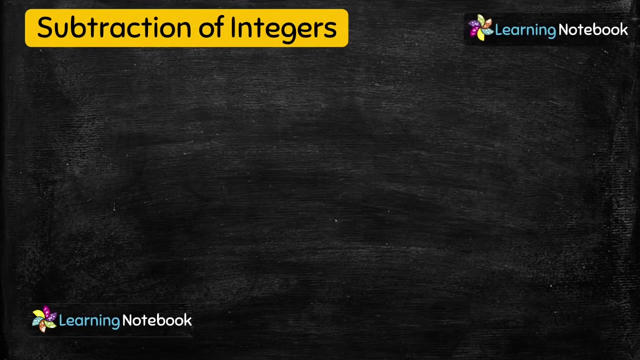 So we will simply add them And copy the negative sign. So 1 plus 4 equals to 5, And we will put the negative sign, So we get the answer as negative 5. Let's do one more example. For example: 5 minus negative 3. 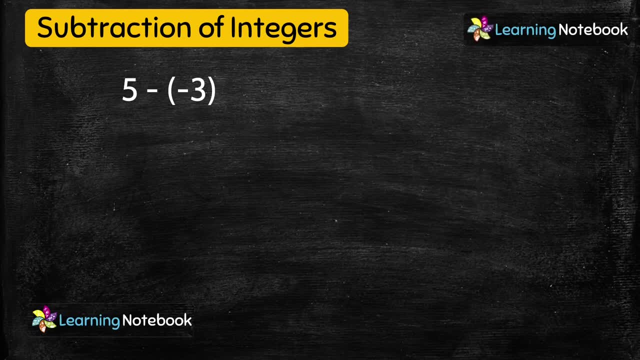 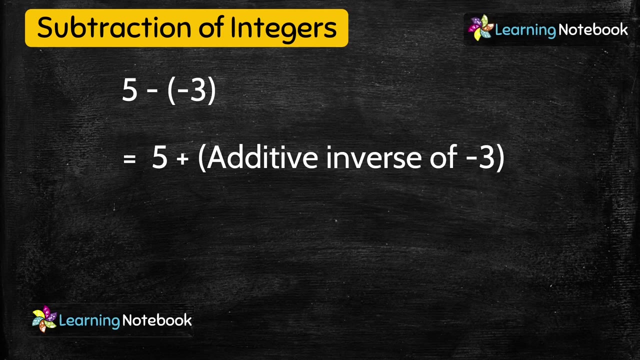 So here we are subtracting negative 3 from positive 5. So to subtract these two integers We will take additive inverse of negative 3, So we get 5 plus additive inverse of negative 3, And we know Additive inverse of negative 3 is positive 3. 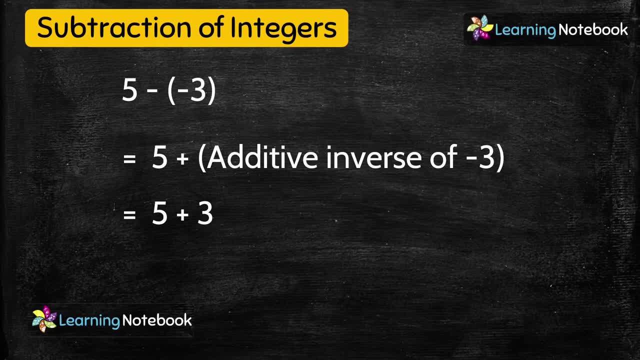 So we get 5 plus 3. Now we will add them, And since both of them are positive integers, We will simply add them and copy the positive sign. So 5 plus 3 equals to 5 plus 3 Equals to 8. 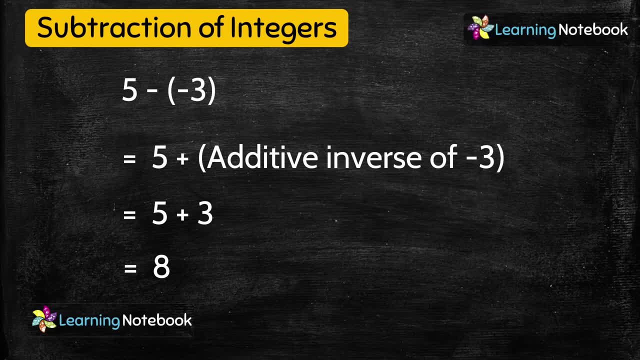 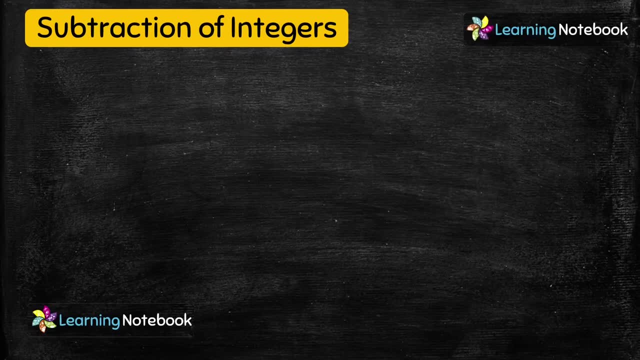 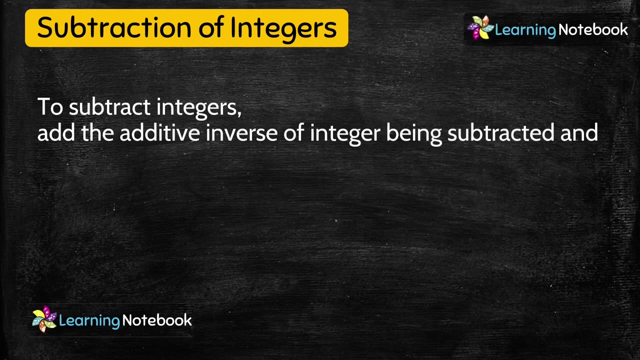 And thus this is our answer. So, students, To subtract integers, We do not need to remember any new rule. We just add the additive inverse of integer being subtracted And follow the rules for addition. Now let's do another example. Let's do subtraction of integers on number line. 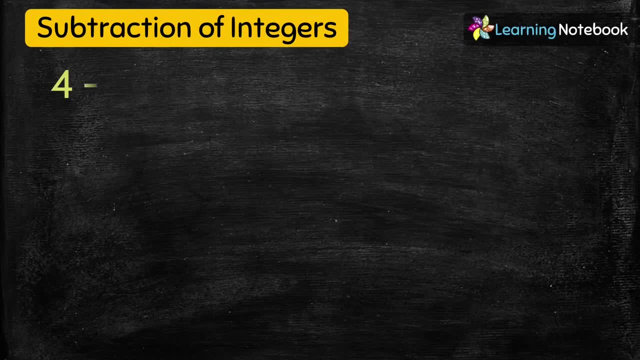 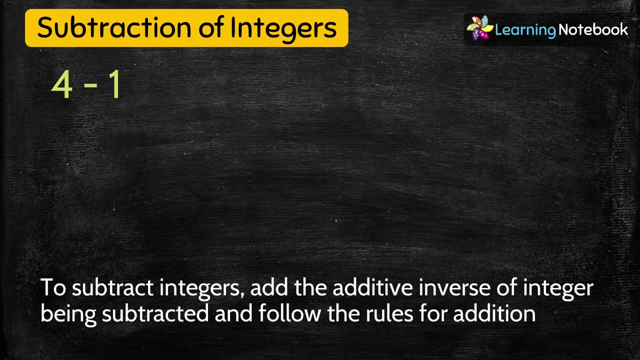 Question is 4 minus 1. So to subtract these two integers, We will add additive inverse of positive 1, And additive inverse of positive 1 is negative 1, So we get 4 plus Negative 1. Now, students, We already know How to add such numbers on number line. 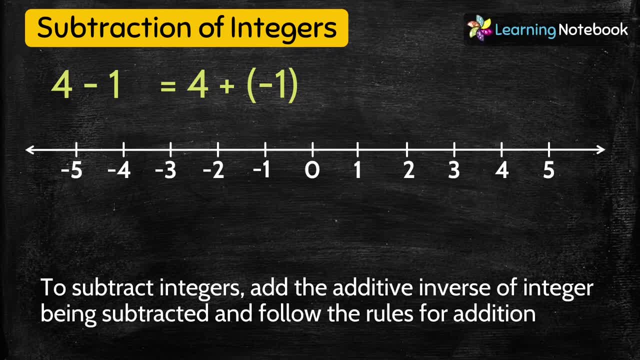 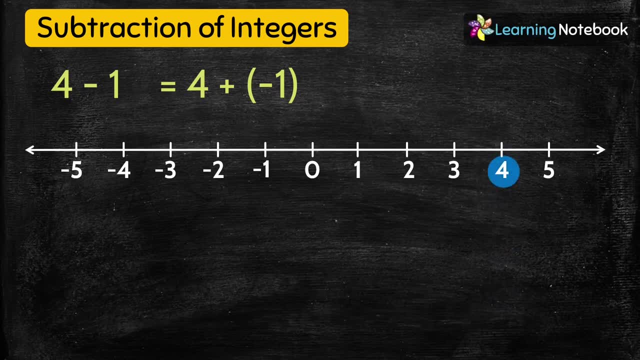 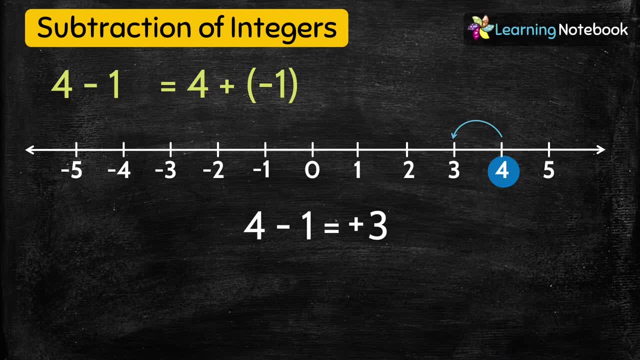 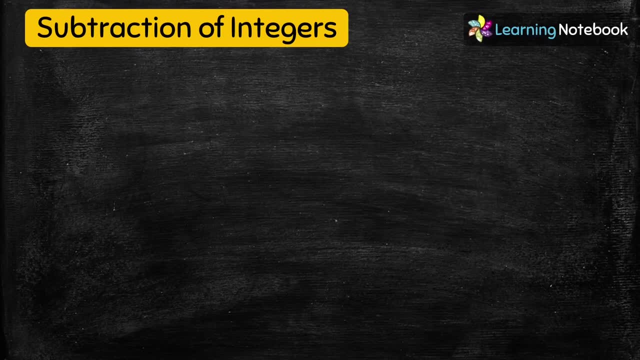 So 4 minus 1 equals to 4. So 4 plus 1 equals to positive 3 Or simply 3. Let's do the next question: 3 minus positive 5. To subtract these two integers Let's add additive inverse of positive 5. 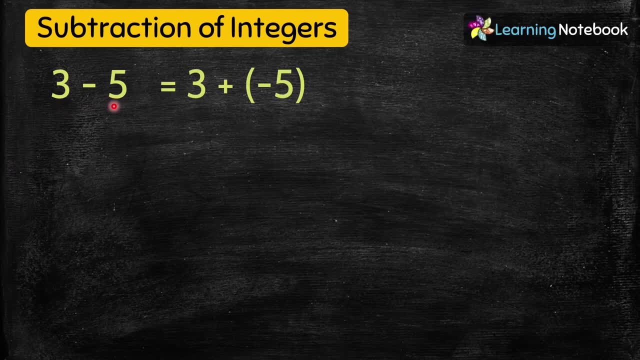 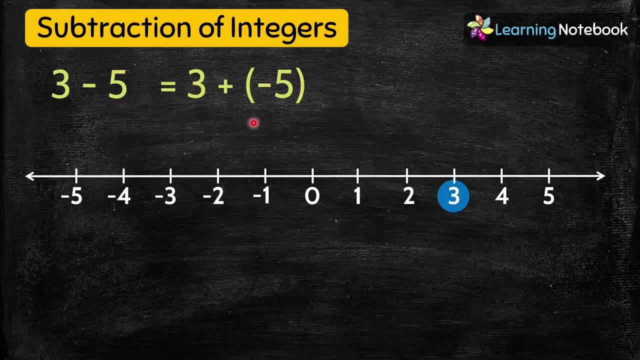 Which is negative 5, So we get 3 plus positive 5 is negative 5, So we get 3 plus positive 5 is negative 5 plus negative 5.. Now here, first number is positive 3 and we are adding negative 5 to. 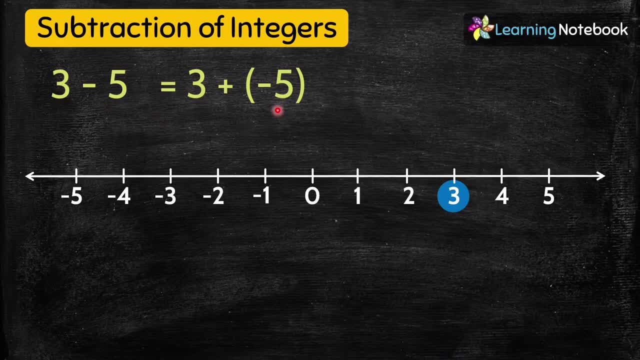 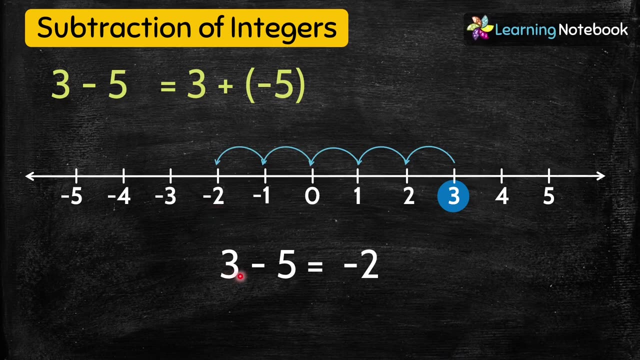 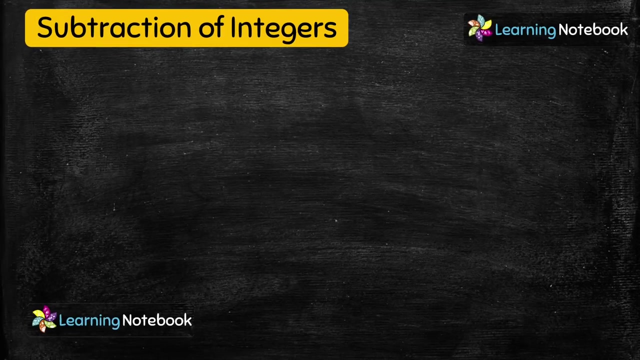 8.. So let's move 5 units to the left of positive 3. We get negative 2.. So 3 minus 5 equals to negative 2.. Let's see the next question: Negative 1 minus positive 2.. So let's add the additive inverse of positive 2, which is negative 2. So we get 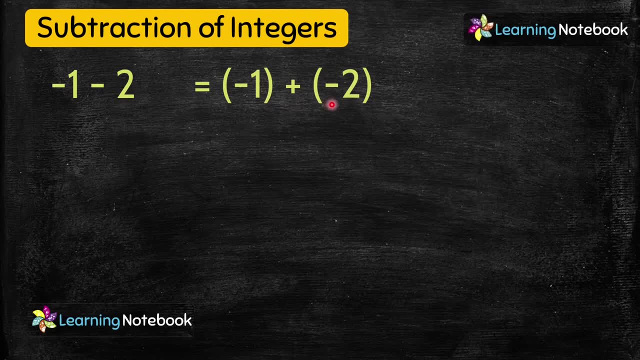 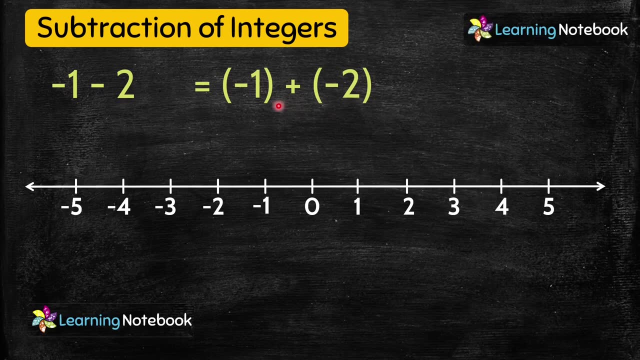 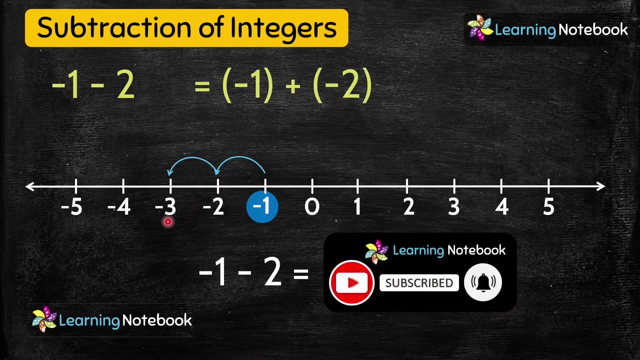 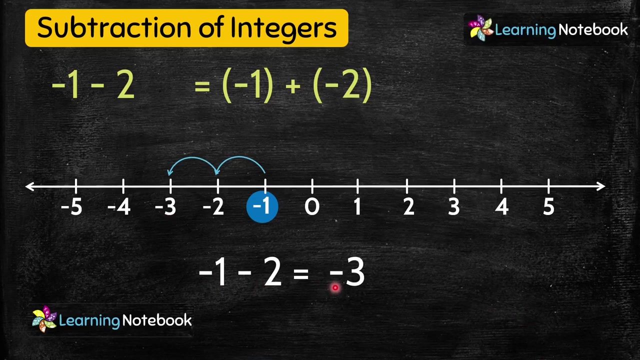 negative 1 plus negative 2.. Now, students, we will add these two negative integers. First number is negative 1 and we are adding negative 2 to 8. So we will move 2 units to the left of negative 1 and we get negative 3.. So negative 1 minus positive 2 equals to negative 3.. 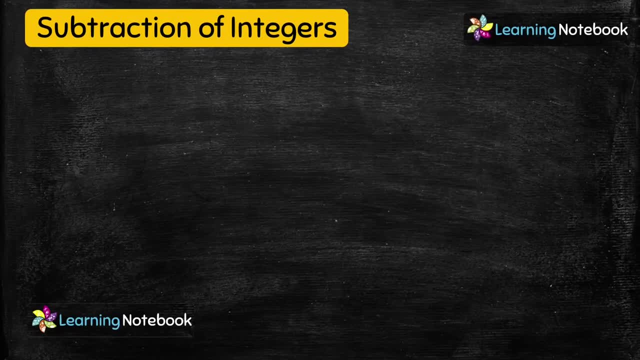 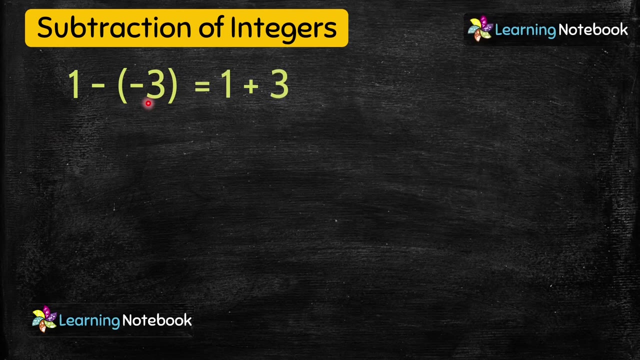 Next question is 1 minus negative 3.. So let's add the additive inverse of negative 3, which is positive 3. So we get 1 plus 3.. Now we will add these two numbers. First number is 1 and we have to add 3 to 8. So let's move. 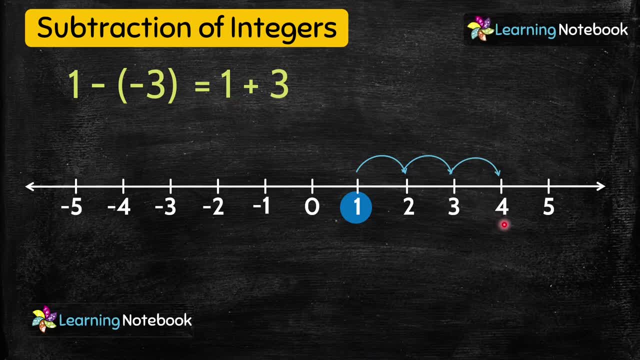 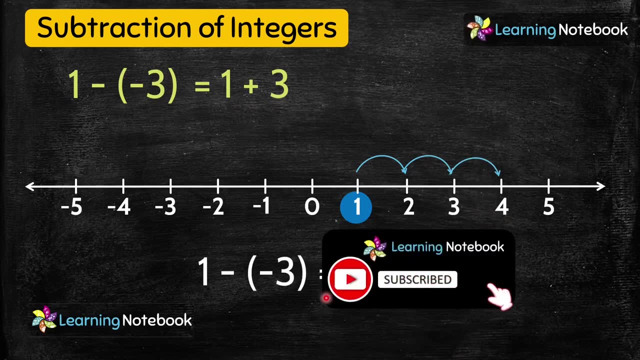 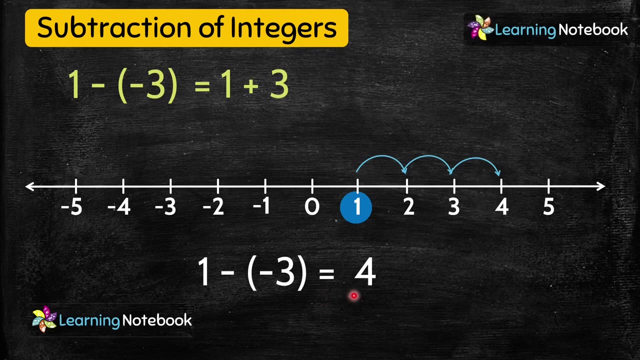 3 units to the right of 1. We get 4.. So 1 minus negative 3 equals to 4.. If you still not have subscribed to our channel Learning Notebook, then do subscribe it and make sure to press the bell icon. 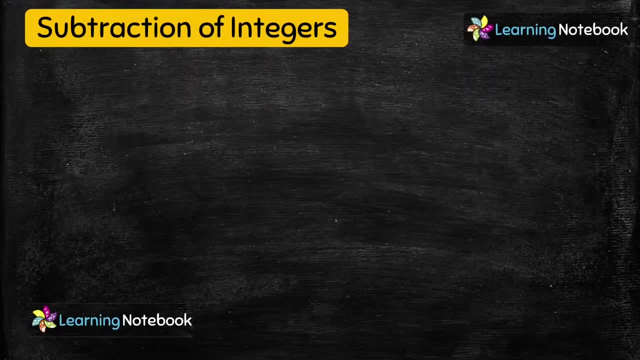 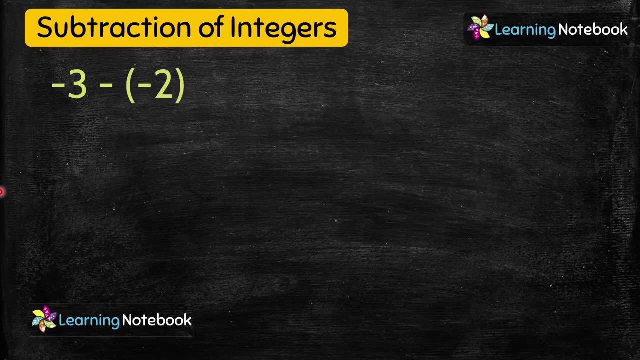 Let's do the last question: Negative 3 minus negative 2.. So let's add additive inverse of negative 2, which is positive 2.. So we get negative 3 plus 2.. Now let's add these two integers. 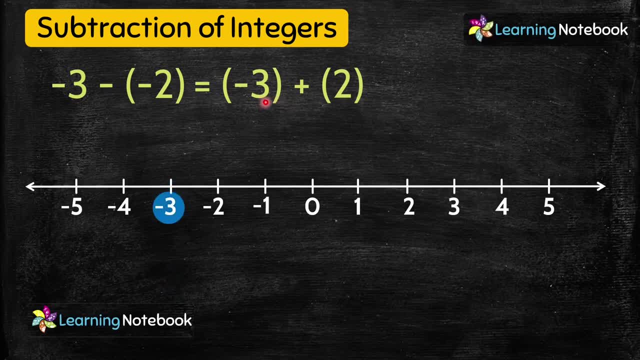 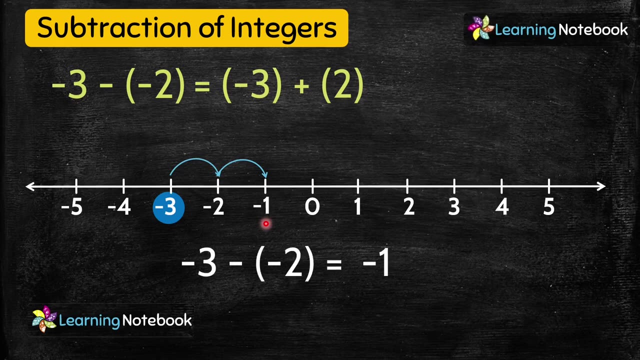 First number is Negative 3 and we are adding 2 to it. So let's move 2 units to the right of negative 3.. We get negative 1.. So negative 3 minus negative 2 equals to negative 1.. 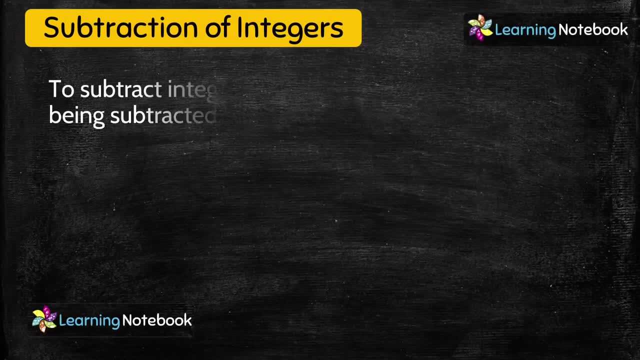 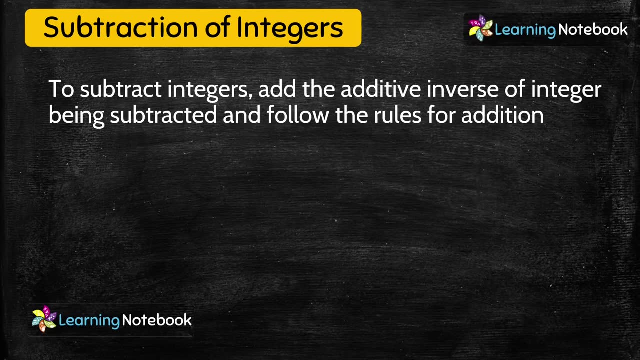 So students do remember That to subtract integers add the additive inverse of integer being subtracted and then follow the rules for addition. For example, 1 minus negative 2 equals to 1 plus 2, which is equals to 3.. 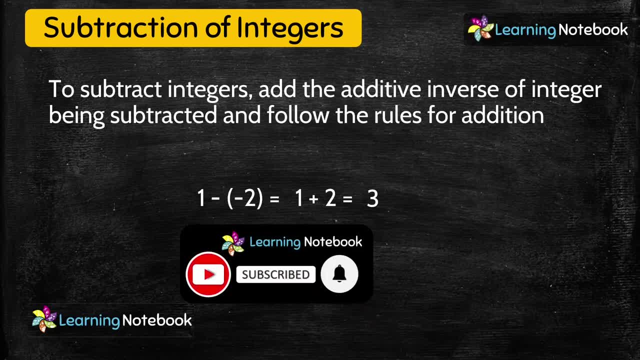 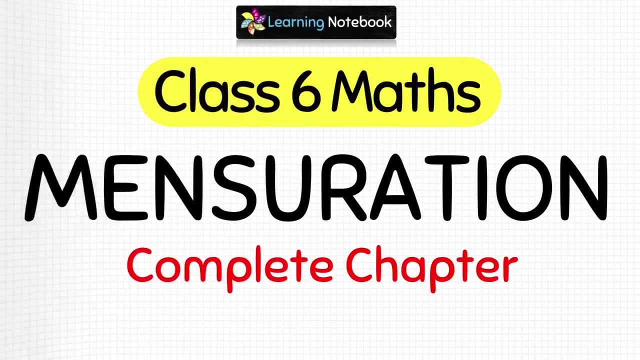 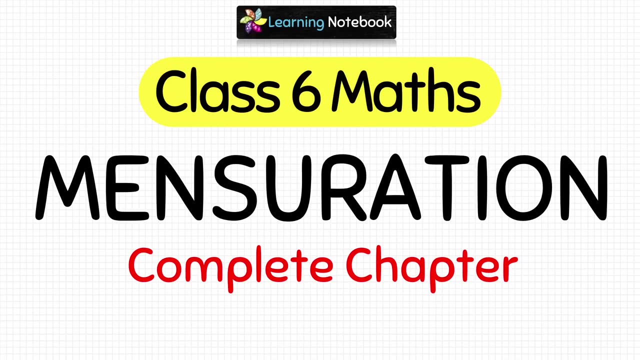 If you still not have subscribed to our channel Learning Notebook, then do subscribe it and make sure to press the bell icon. We also have a separate video on complete chapter of mensuration for class 6.. In this video you can learn about what is perimeter, what is area. 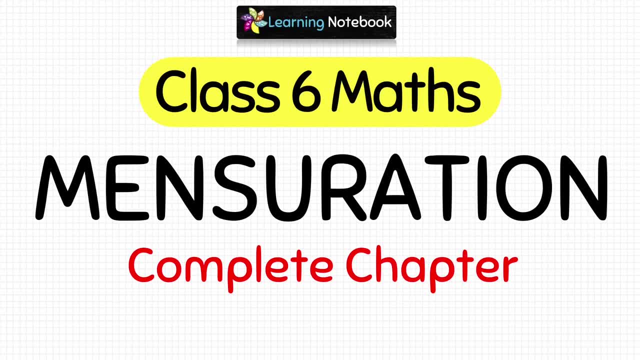 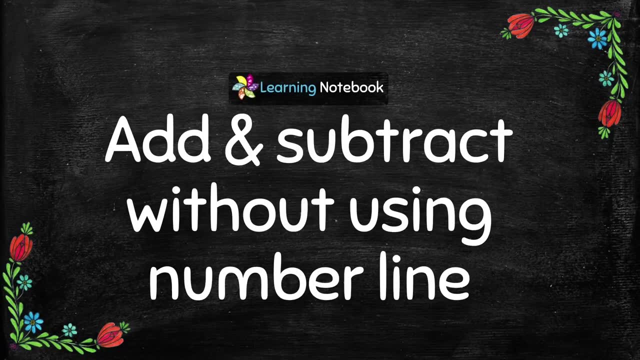 and how to find perimeter and area of rectangle and square. Students, you will find the link to this video in the description box. Now let's add and subtract without using number 9.. Now let's add and subtract without using number 9.. 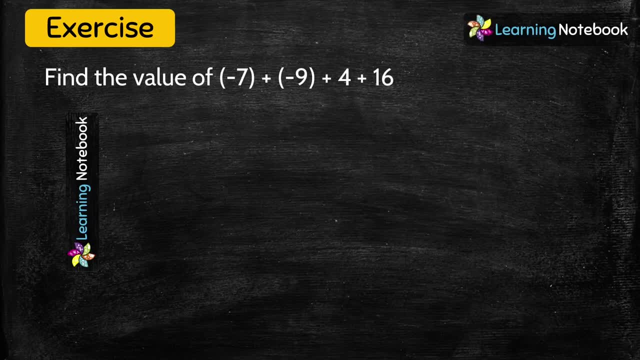 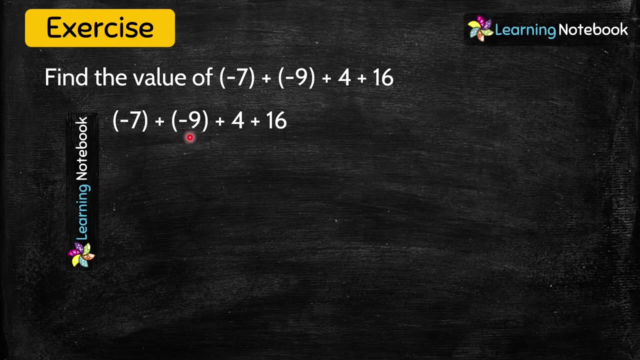 Question is: Find the value of negative 7 plus negative 9 plus 4 plus 16.. So here, students, we are given with 2 negative Integers and 2 positive integers, So let's first add these 2 negative integers. 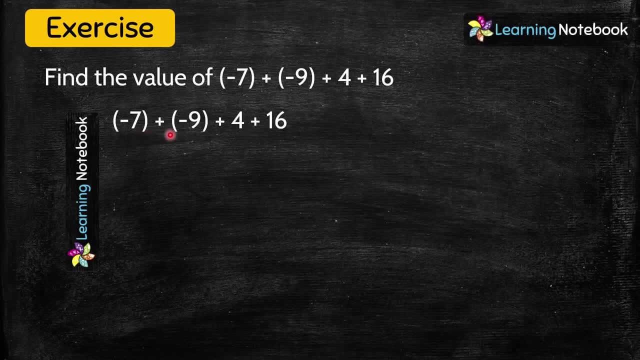 We know when we are adding 2 negative integers, we simply add them and copy the negative sign. So 7 plus 9 equals to 16, and we will copy the negative sign, So we get negative 16.. Now let's add these 2 positive integers. 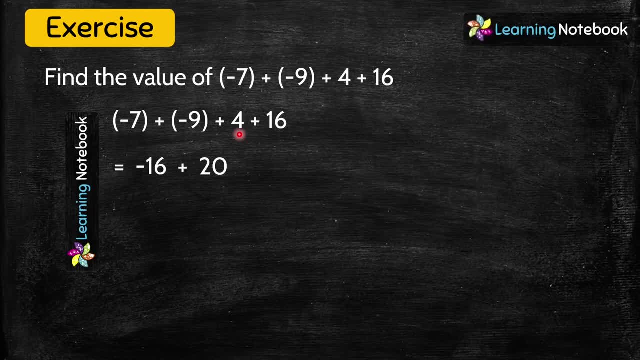 Again, we will simply add them and copy the positive sign. So 4 plus 16 equals to 20.. Now we have got 1 negative integer and 1 positive integer And to add such integers of opposite sign, we subtract them and copy the. 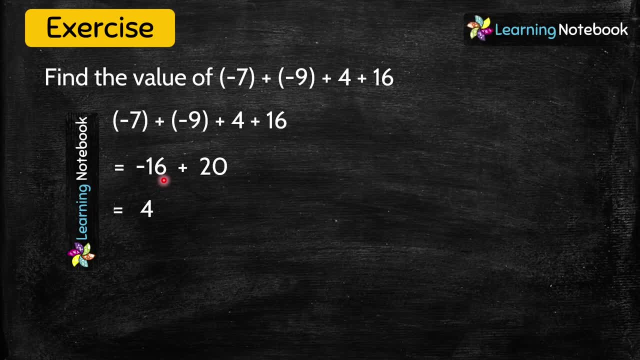 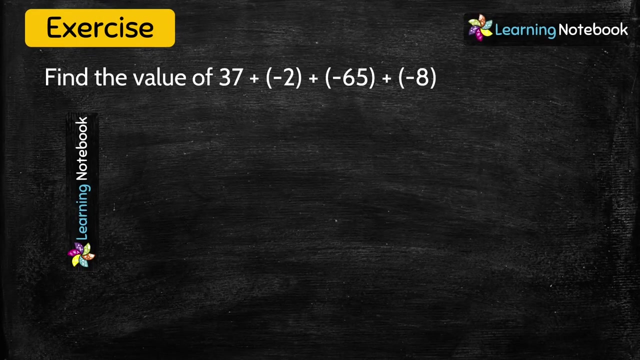 Integers Copy the sign of the bigger number. So 20 minus 16 equals to 4, and bigger number is 20, which has positive sign. So we get the answer as positive 4 or simply 4.. Let's see the next question. 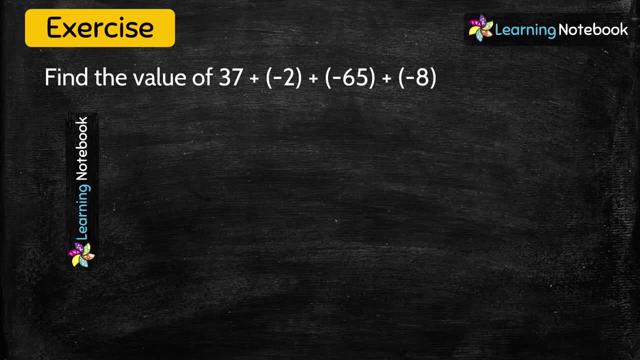 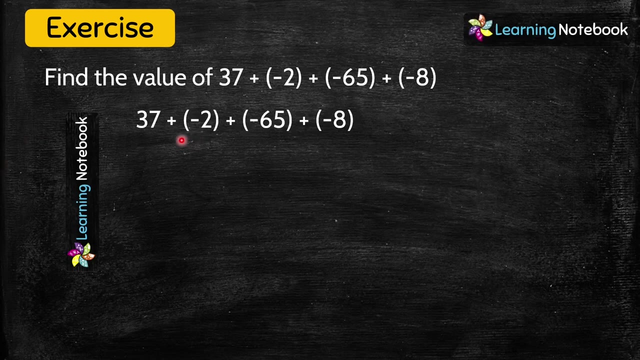 Find the value of 37 plus negative, 2 plus negative, 65 plus negative 8.. So, students, here we are given with 1 positive integer and 3 negative integers. So let's first add these 3 negative integers, So 2 plus 67.. 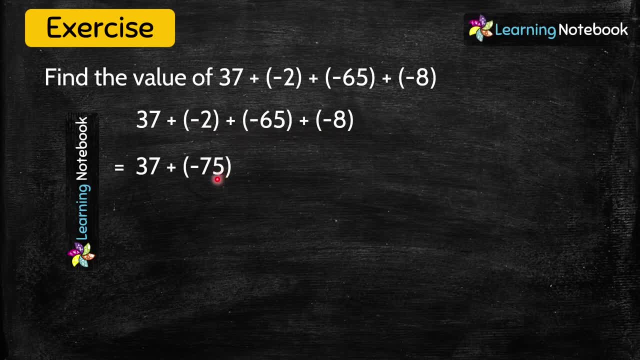 55 plus 8 equals to 75, and we will copy the negative sign So we get negative 75.. So now we have 1 positive integer and 1 negative integer. So let's subtract them: 75 minus 37 equals to 38.. 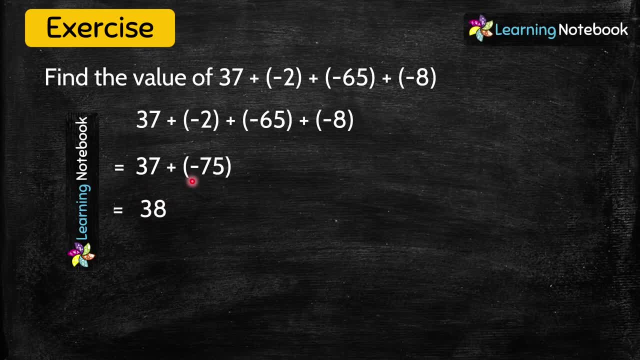 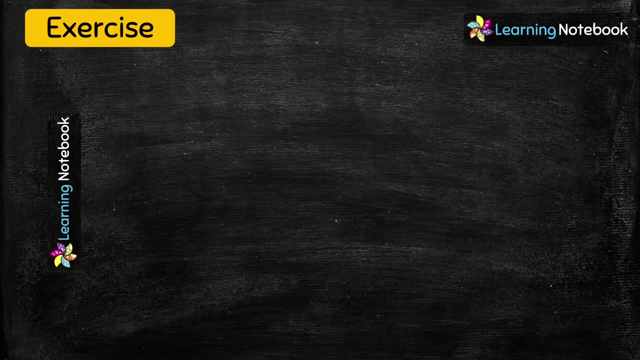 And we will copy the sign of the bigger number, which is 75, and its sign is negative. So we get the answer as negative 38.. Next question is: find the value of negative 10 plus negative 9 minus negative 7.. So here, students, first we will: 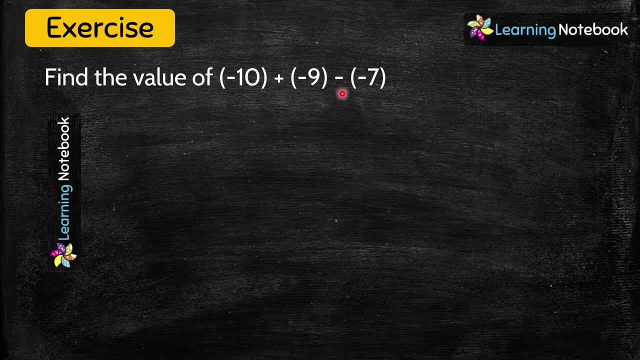 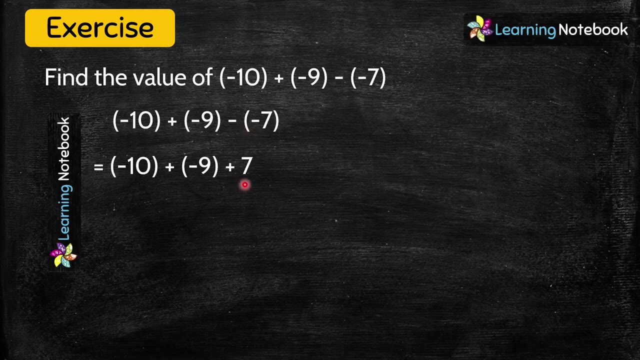 We will do subtraction. So to subtract we will add the additive inverse of negative 7. And additive inverse of negative 7 is positive 7. So we get negative 10 plus negative 9 plus 7.. Now let's add these 2 negative integers. 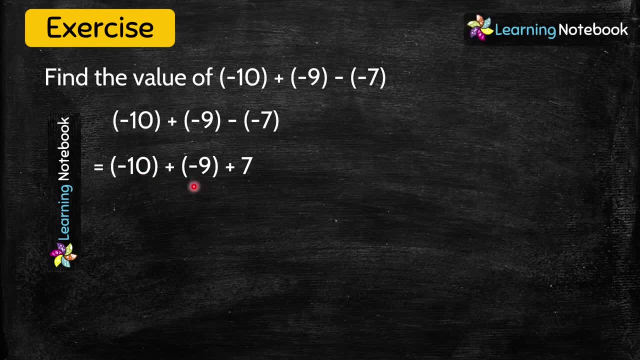 So 10 plus 9 equals to 19 and we will put the negative sign. So 10 plus 9 equals to 19 and we will put the negative sign. Now we are left with 1 negative integer and 1 positive integer. 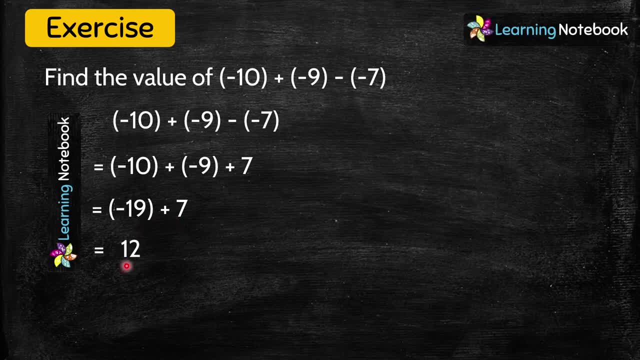 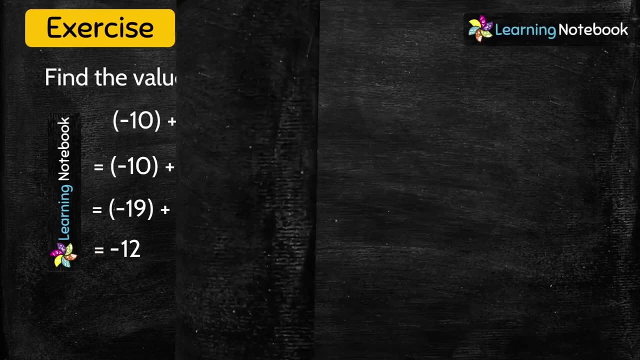 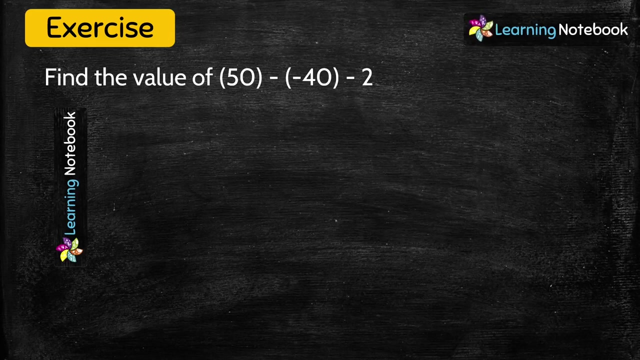 So we will subtract them- 19 minus 7 equals to 12, and we will copy the sign of bigger number, which is 19.. So we get the answer as negative 12.. Now let's do the last question: Find the value of 50 minus negative, 40 minus 2.. 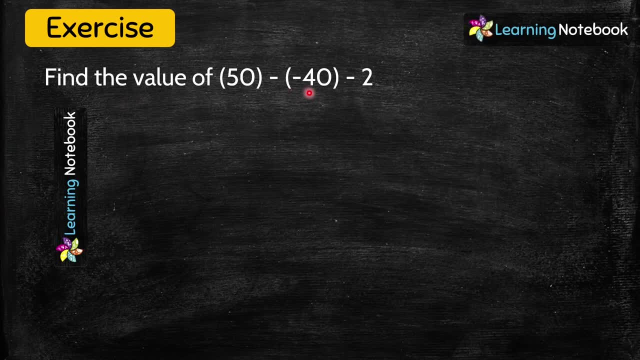 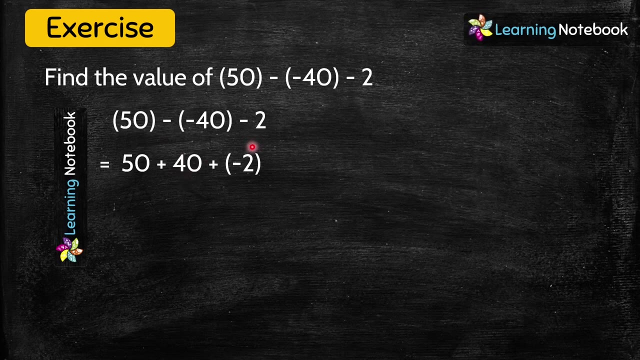 So here we are, subtracting negative 40 and positive 2.. So let's add their additive inverse. Additive inverse of negative 40 is positive 40. And additive inverse of positive 2 is negative 2.. So we get 50 plus 40 plus negative 2..